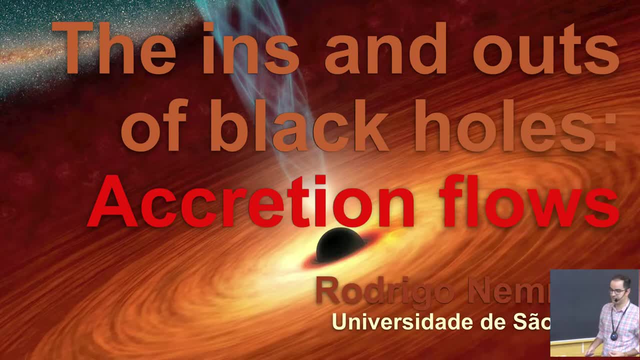 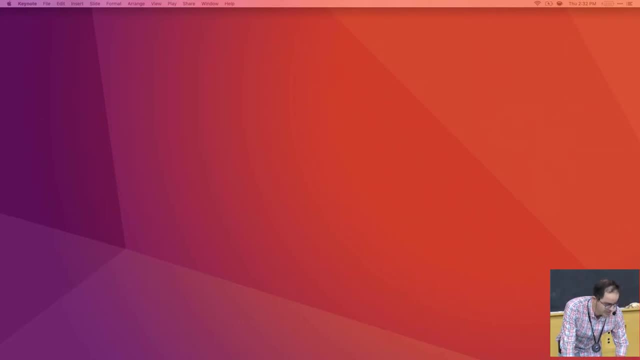 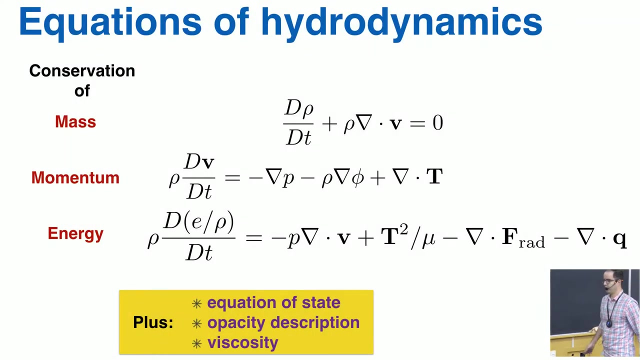 and therefore have a global view of the ins and outs of black holes, As we stopped yesterday, which was We had an overview of the conservation equations for the mass, the momentum and the density in fluids: The conservation equations. 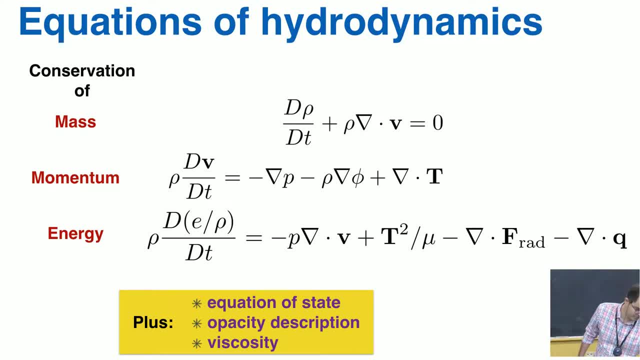 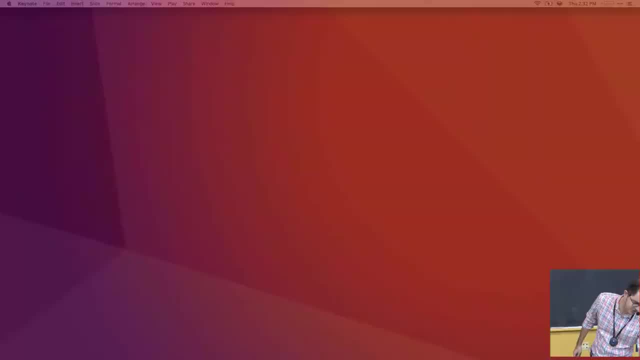 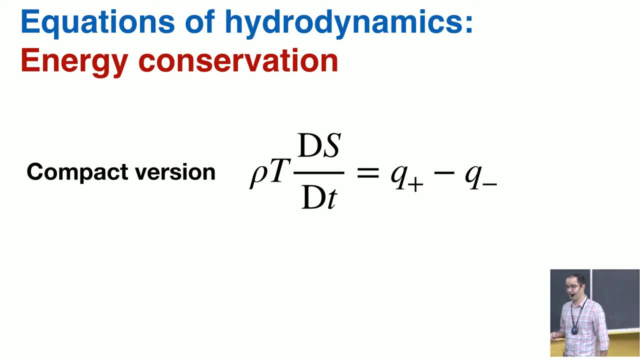 of hydrodynamics, the Newtonian conservation equations, And then we saw a very we saw a modified version of the energy conservation equation which will be relevant to to have a broad, unified view of accretion disks. 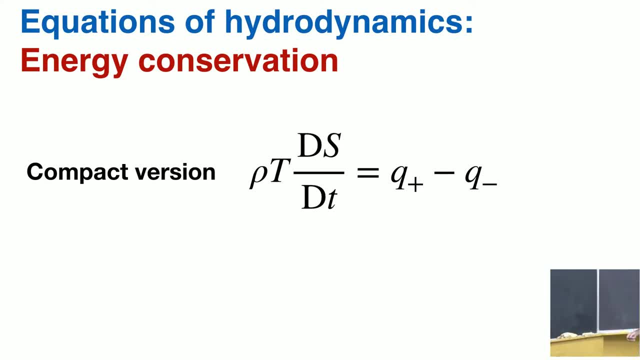 So this is, as I was saying yesterday, this is the energy conservation equation in a slightly different and more compact version, where you have the Lagrangian derivative of the entropy of the fluid, which is equal the heat generated in the fluid, minus the cooling, the energy lost by any sort of cooling. 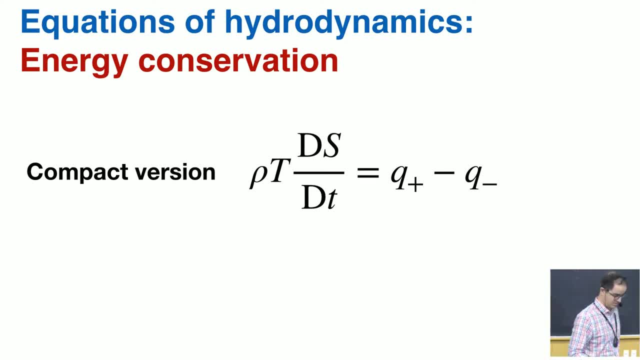 One second. Somebody. has somebody retained the USB receiver here? Ian Sasha, did you keep the receiver? No, Yeah, Okay, Gone with the wind Right. Ah, there you go, OK, thank you. 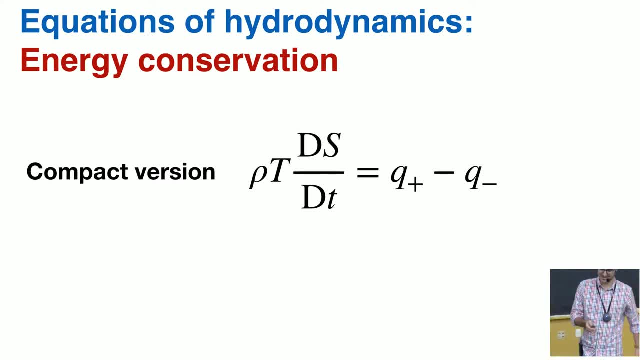 It was accreted back. OK, no problem, Right, so this compact version of the energy conservation equation we can simply understand as a statement that the heat energy must go somewhere. Don't worry, it's not a big deal, OK. 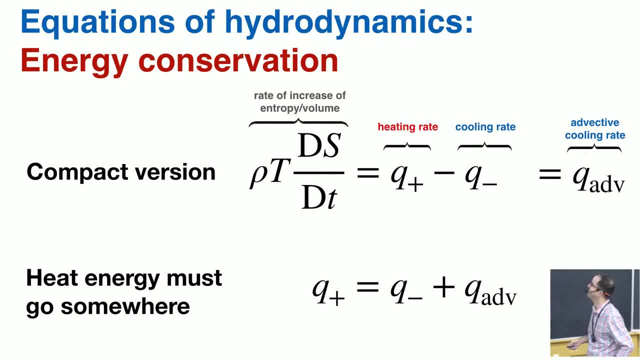 Don't worry, Stay cool, take it easy. So this equation really means that the heat energy generated by viscous dissipation- sorry, the key plus- it must go somewhere. So part of it goes into radiative cooling, Part of it is advected with the fluid. OK, 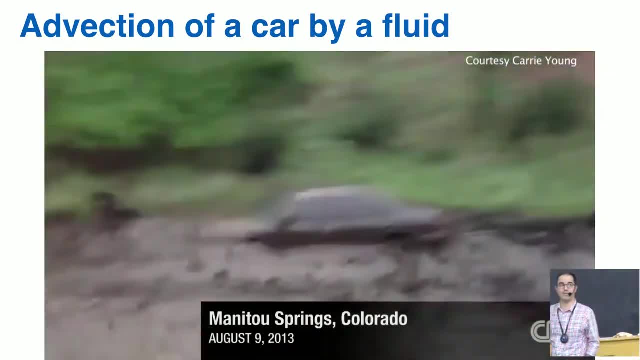 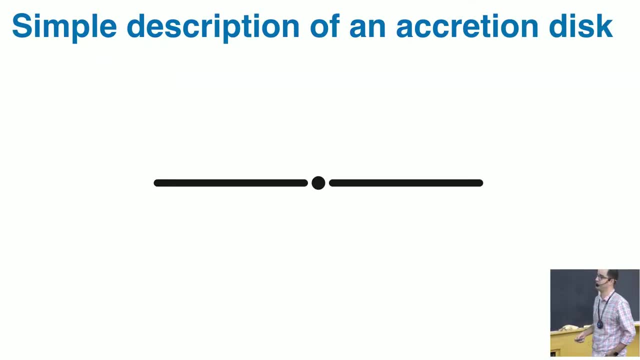 And then you understood what is advection by this simple example of the advection of a car by a fluid. So now we can proceed and have a very simple description of an accretion disk. OK, The Navier-Tokes equation is very complicated, right? 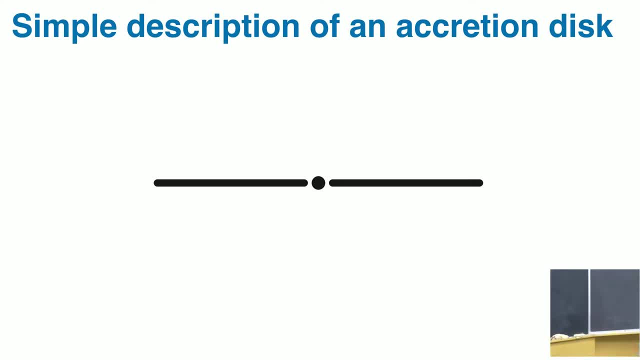 And we, as theorists, we are trying to simplify our view of the universe as much as possible. So let's characterize an accretion disk by right now. of course there is the mass of the black hole, the gravity parameter, so the mass and the spin. 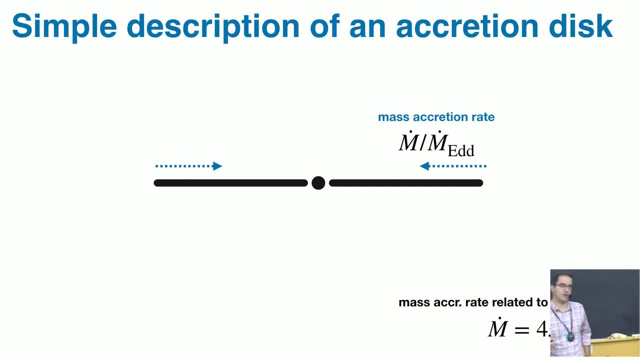 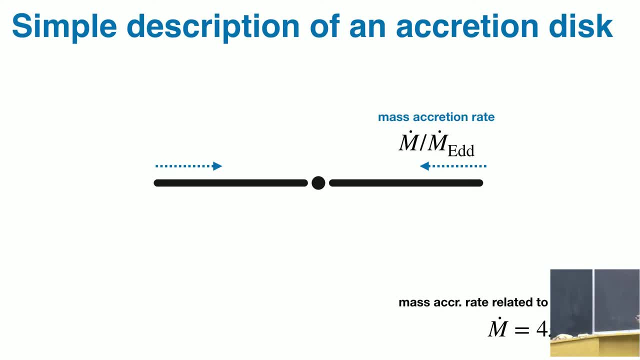 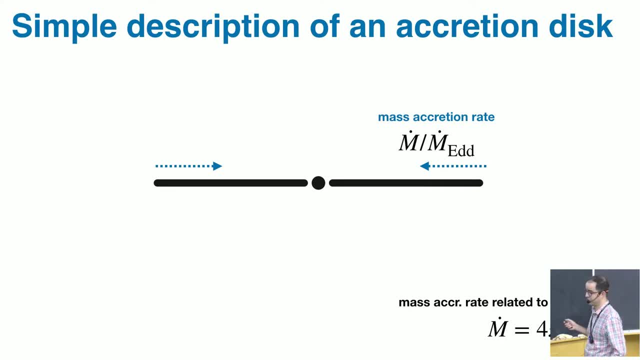 through the Addington rate. as we learned yesterday the definition of the Addington luminosity and the Addington accretion rate, We can think of the Addington accretion rate as a limiting accretion rate, a sort of a scale. 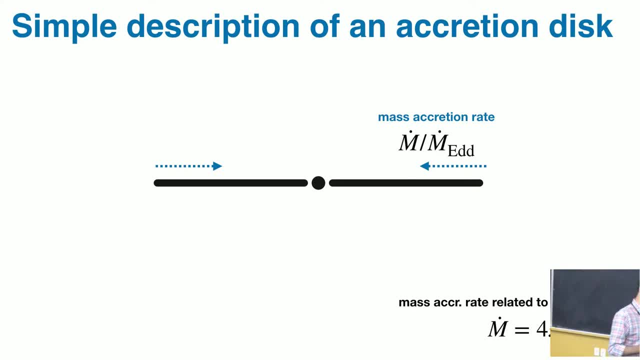 that whenever this ratio here goes close to 1, you are nearing trouble in your accretion, accretion physics, because you're reaching the maximum limit with which you can feed the black hole. if you try to feed the black hole in principle in a 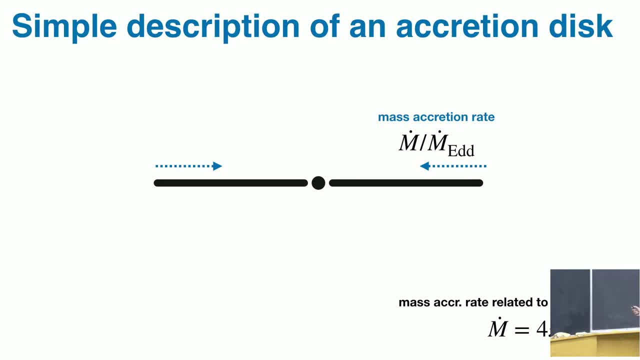 spherically symmetric way above a ratio of this ratio above one, then your black hole might start refusing further accretion of material. so this is the first number. the accretion rate is really related to the density. okay, we can. we can work with the continuity equation and we can find out that the 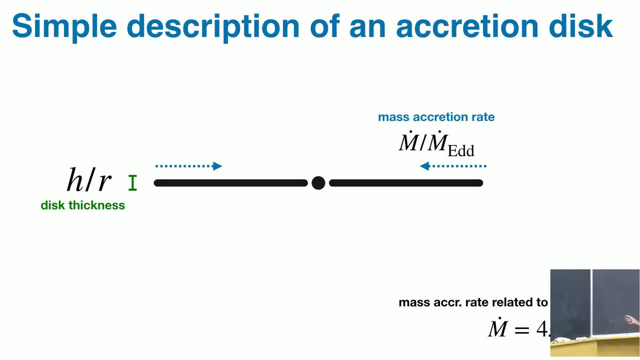 this value is parameter here. the accretion rate is a conserved quantity of the fluid of the accretion disk. so the accretion rate is really related to the density of the fluid. so whenever we increase or decrease the accretion rate, we are increasing or decreasing the density. 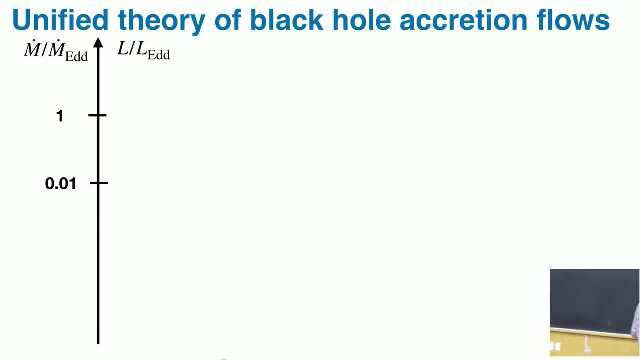 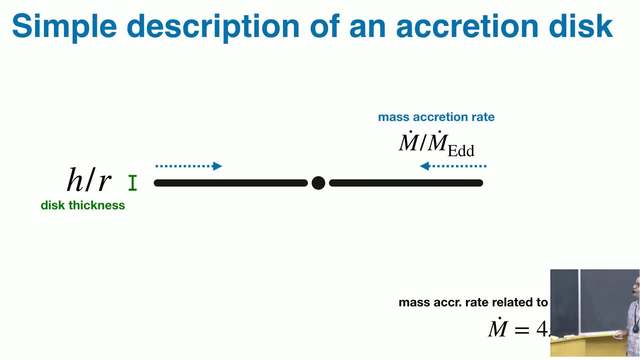 of the gas. okay, and the second number that we will pay attention to, which is really related to the global, global properties of the disk, is the disk thickness, which is the rate as to the radius. okay, so whenever the disk is thick, this ratio here will go up. if it, if it is very thin, this ratio will. 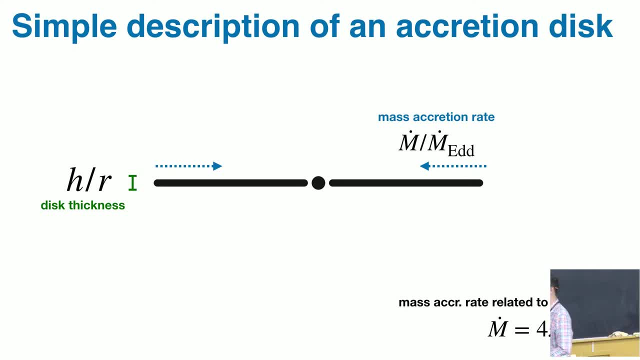 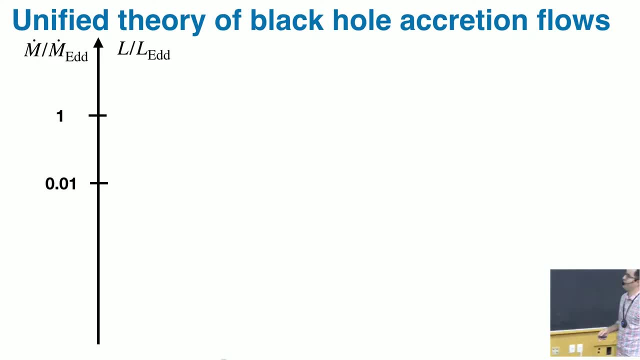 be much smaller than one because the thickness is much smaller than the radius of the, the radius where you are considering the disk. so now we are ready to try to have a global, unified theory of a black hole accretion disks. so those actors show the ratio of the accretion rate to the. 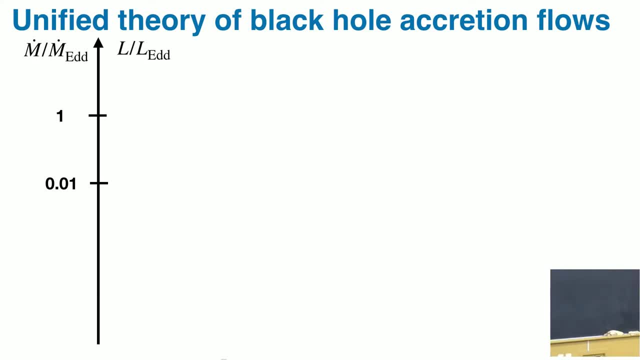 addington accretion rate. it is more or less the same thing as the ratio of the luminosity release by the accretion disk over the addington luminosity. okay, so the The first solution, the first regime of black hole accretion happens, occurs for ratios. 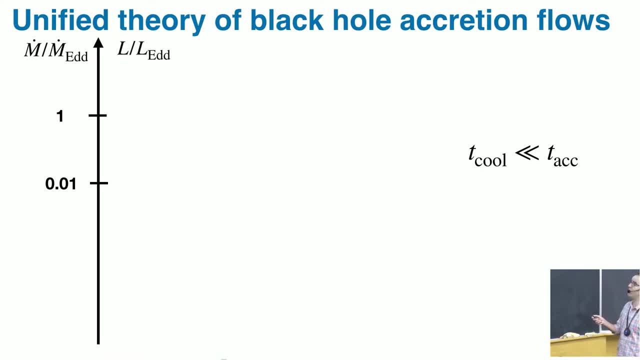 for the accretion rate over, adding to an accretion rate between 1 and 0.01, in other words 1%. So in these conditions what happens is that you have high densities of the accretion disk, So the cooling time the disk has a high density. 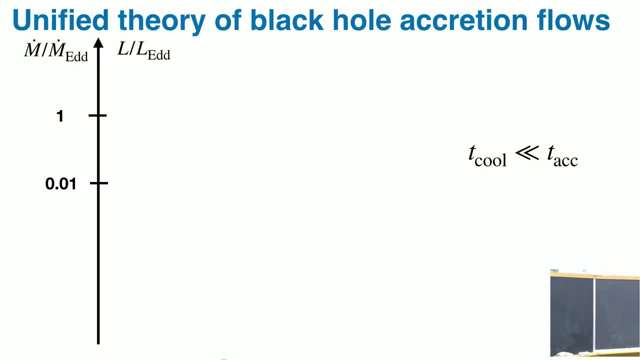 The electrons which radiate. they are interacting strongly with the protons through Coulomb collisions. So the protons get the viscous heat energy and they transfer to the electrons via Coulomb collisions. If you have high densities, the electrons get very rapidly the energy from the protons and they radiate it away. 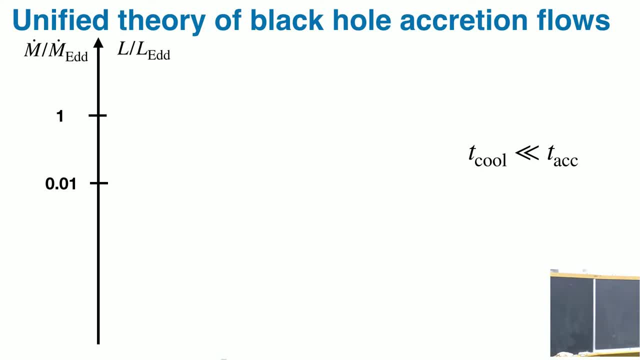 So the cooling time is much smaller than the time it takes for a portion of the disk to fall into the black hole. In other words, the disk will try to get rid as fast as possible of its heat energy. In other words, the cool, the radiative cooling time term is much more important than the advection cooling term. 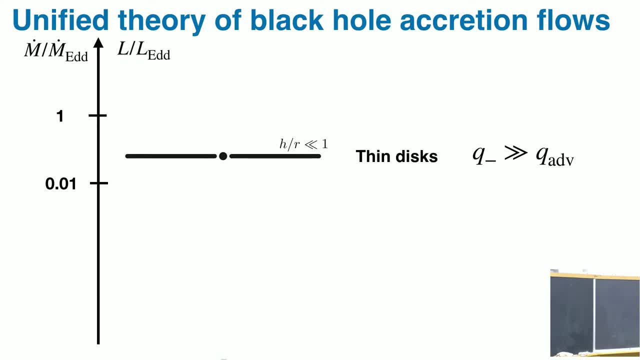 In these conditions, what happens with the accretion disk is that the disk cools very rapidly. There is not a lot of pressure to support the disk, So the disk collapses. The disk collapses into a thin, quasi-Couplegian disk, what we call thin disk, with a very small height. 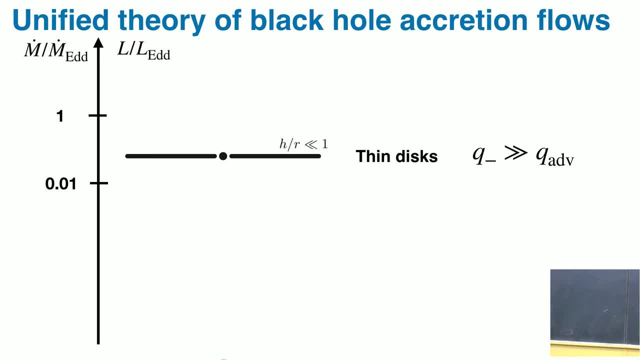 Very thin disk as we call for this range of accretion rates. Now if you start decreasing the accretion rate, the density also goes down. And because the density goes down, the interactions between electrons and protons they get. they start becoming rare. 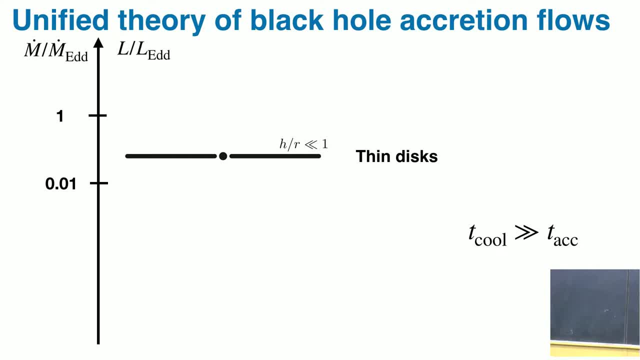 So the protons will get the heat energy from viscosity. They get the heat energy from turbulence, But the electrons will not receive that viscous energy by Coulomb collisions. All of this is related to the microphysics of the disk. That's why I'm talking about the microphysics. 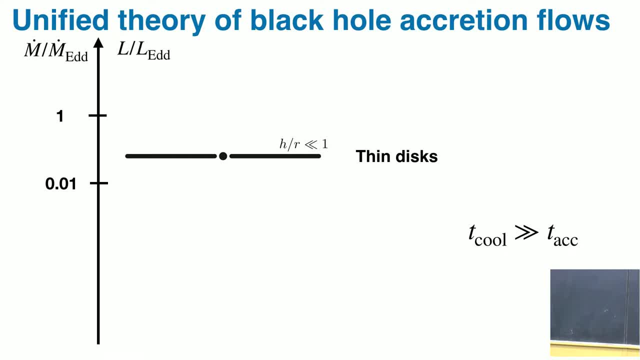 So when you decrease the accretion rate, you go down in this axis here. you decrease the density, The cooling time starts getting very big And in fact the cooling time gets bigger than the time it takes for the gas to be accreted by the black hole. 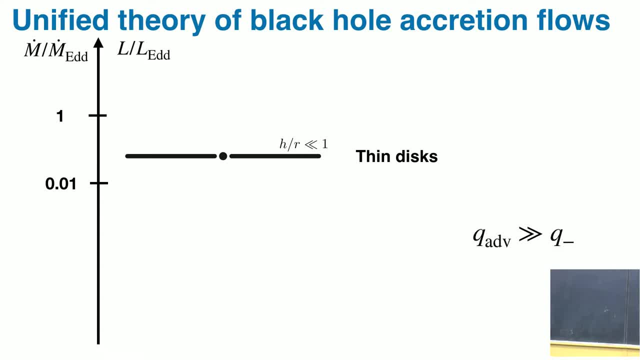 In other words, the advective cooling ratio is much bigger than the time it takes for the gas to be accreted by the black hole. In other words, the advective cooling ratio is much bigger than the time it takes for the gas to be accreted by the black hole. 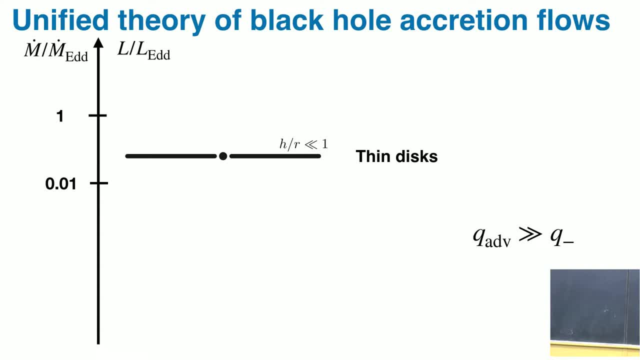 When the advective cooling ratio gets bigger than the radiative cooling rate? When the advective cooling ratio gets bigger than the radiative cooling rate, what happens now is that the heat energy will not be released by radiation, So the gas will store the heat energy. 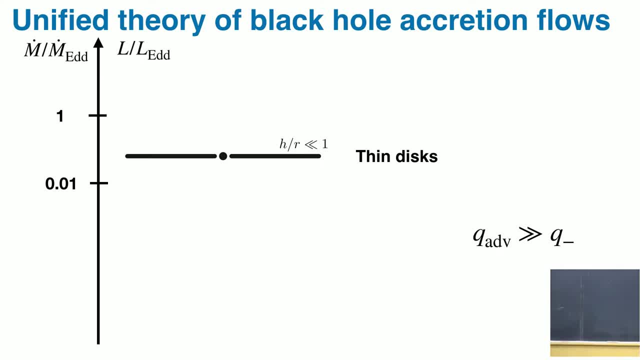 And it will keep storing and hitting energy and it will inflate like a balloon. The accretion disk will inflate like a balloon And it will reach a new vertical hydrostatic equilibrium configuration where they will become very thick because of the high thermal pressure. 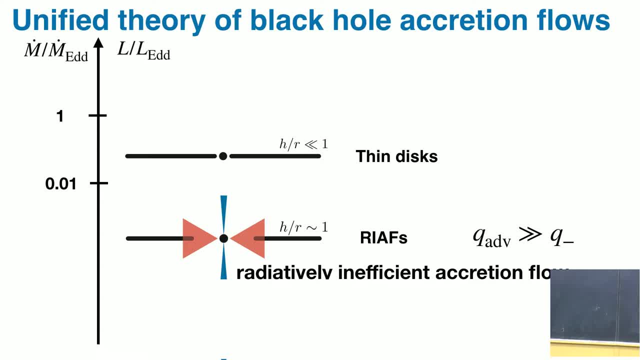 And so the h over r will get big, will get close to 1.. And in this case, what happens here is that the disk, instead of releasing the heat energy as radiation, it stores the heat energy, thermal energy, and gets very thick, almost like a balloon. 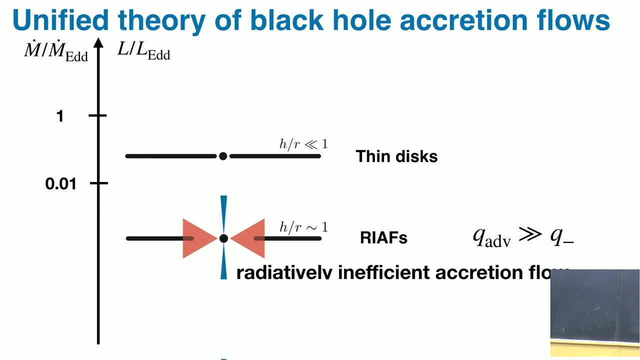 And we call it a radiatively inefficient accretion flow, because it's a very inefficient radiator, this kind of accretion disks with low accretion rates. Now, if we keep decreasing, look, there is something interesting happening here. 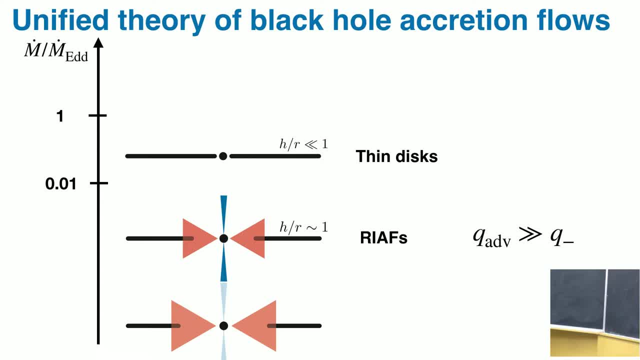 I'm showing you also this blue thing, which is really the jet from the black hole that I will talk. I will describe the physics of the jet in the next lecture. I will not talk right now about the physics of the jet, But look, so you can keep playing this game. 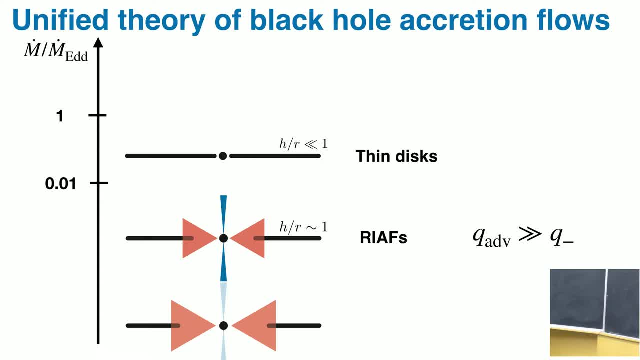 if you're feeding a black hole, if you have a nice black hole that you love and share, If you're home, if for some reason you don't like your black hole, you can starve your black hole And then the accretion disk will bloat and will get thicker. 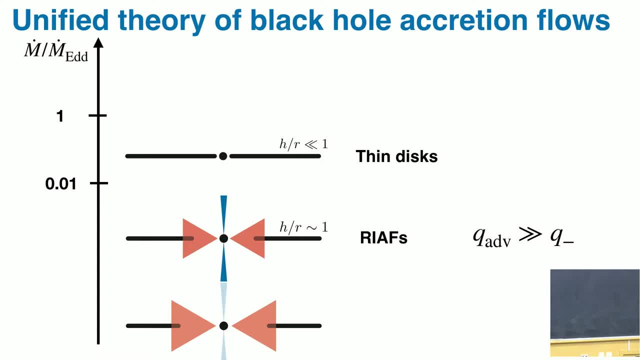 and thicker and thicker. We believe that this is the general configuration of the supermassive black hole at the center of our galaxy: an underfed, starved, almost starved black hole, but not completely starved. On the opposite end, what happens? 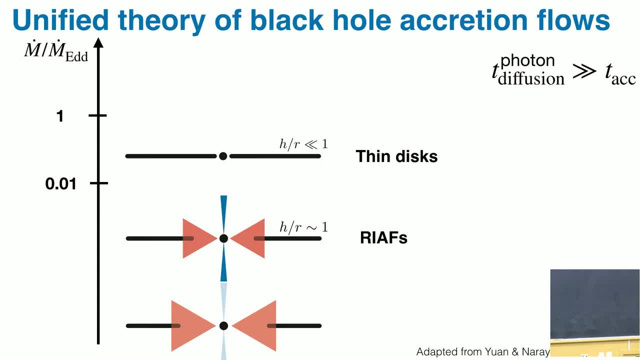 if you try to overfeed a black hole? What happens? if now you want to feed your black hole, You bring your black hole on a date to a Brazilian churrascaria and it eats a lot, And it eats so much that it eats rest mass energy. 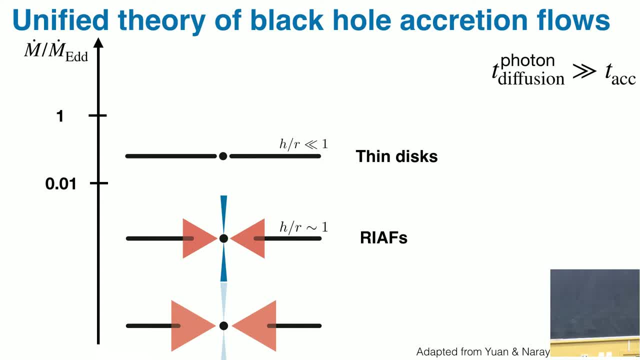 above the Eddington limit. What happens in this case? The thing is, this is possible because we derive the Eddington luminosity limit for a black hole, For a spherically symmetric accretion, But in reality it will have violations. 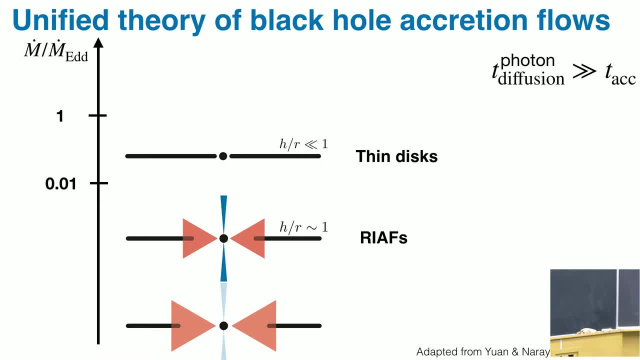 to the spherically symmetric accretion, And so accretion above the Eddington limit. it is indeed possible, And this is the least well understood solution to the black hole accretion disks. So in this case, what happens is that the disk 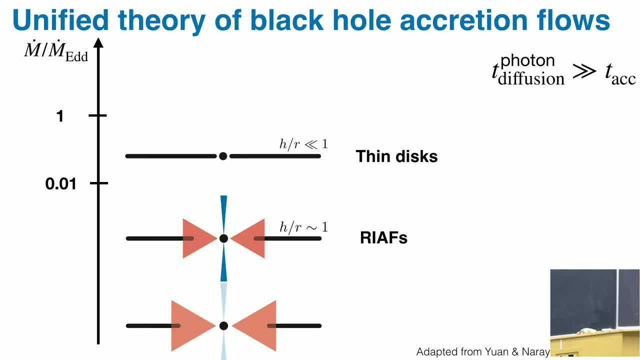 has a very high density So it is basically opaque. So photons will diffuse inside the gas and take a very long time to leave the gas. So the photon diffusion time scale is now larger than the accretion time scale. So now radiation pressure will inflate your accretion disk. 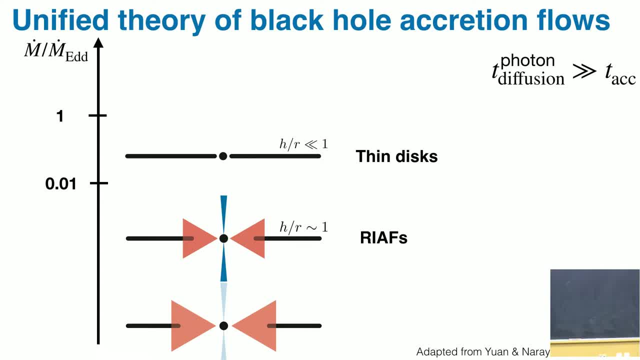 like a balloon, Not thermal pressure, radiation pressure. And now we will have what we call the super Eddington accretion disks, which we understand very little, both from the analytical point of view and from the point of view of general relativistic MHD. 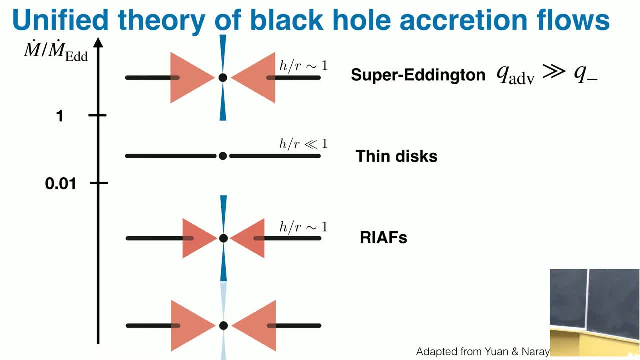 radiation numerical simulations. And this is what happens with the radiative efficiency. Remember the radiative efficiency that we mentioned already during the lectures. This is the power output of your accretion disk. It is related to the mass, to the rest: mass energy. 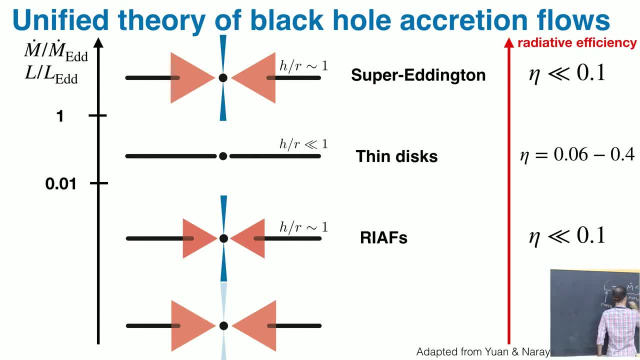 of your fuel supply to your black hole, And this is the radiative efficiency of your accretion disk. This is what we think happens with the radiative efficiency as a function of this ratio, m dot over m dot Eddington, So the highest efficiency is achieved. 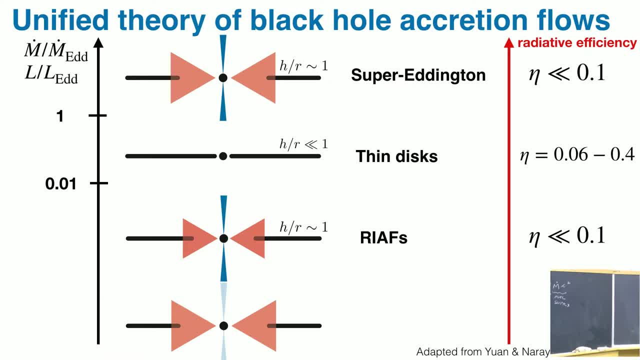 for thin accretion disks, For super Eddington disks, they don't like to radiate, So the efficiency, we believe it's very low. And for static, For black holes, the efficiency is also very low, basically due to the relation between the microphysics. 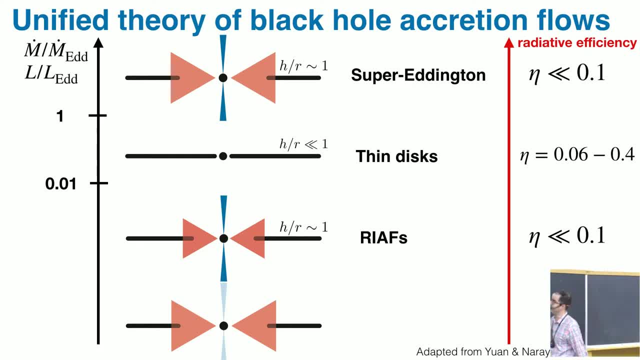 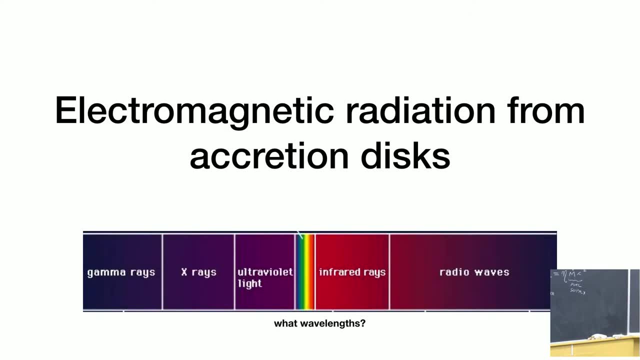 of electron heating and the density of the gas. So now we have a unified theory of black hole accretion disks. The next question is where, if you are designing an astronomical mission, where in the electromagnetic spectrum would you try to search for the signatures of the presence? 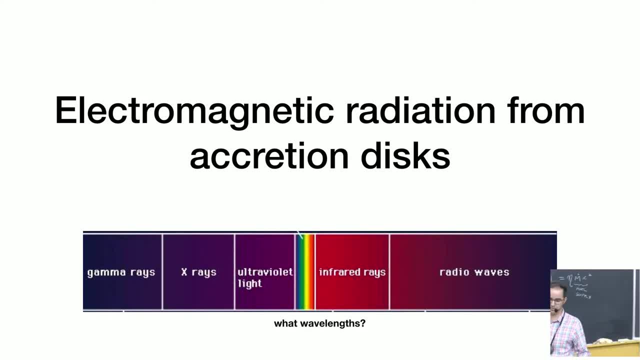 of these accretion disks around black holes? And, if so, how would you do that? Well, first of all, you would have to do a lot of research, and you would have to do a lot of research, and you would have to do a lot of research. 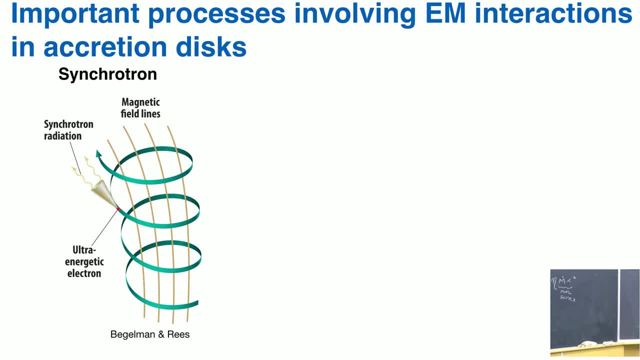 to find out what the difference is between the black holes and the particles in the universe, Then now we must understand how matter couples with radiation in these gases flowing and spiraling towards black holes, And so here is a picture of some of the important processes. 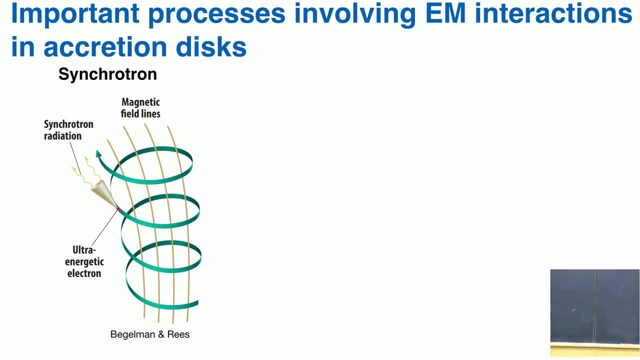 of the electromagnetic interactions with matter in accretion disks. These electrons are moving around these magnetic field lines. So you have, this is the Larmor radius of the electron moving in the magnetic field And you have this accelerated electron spiraling in magnetic field lines. 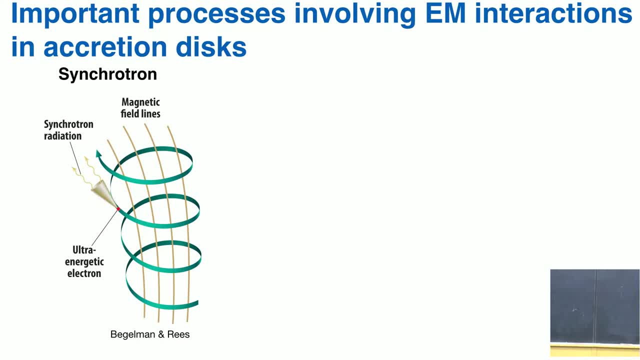 And so you have what we call the characteristic synchrotron radiation from these accelerated charges moving in spirals following the Larmor radii. So we expect to see synchrotron radiation. We expect also something called complex radiation. We expect also something called quantum scattering, which is electrons. 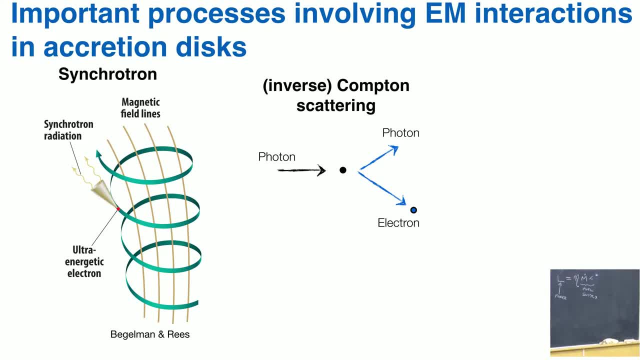 are colliding with photons. You have in the accretion disk a rich gas of particles with a rest mass which is not zero, And you have a relativistic gas of radiation with a rest mass of zero. So the photon field will interact with the electron. 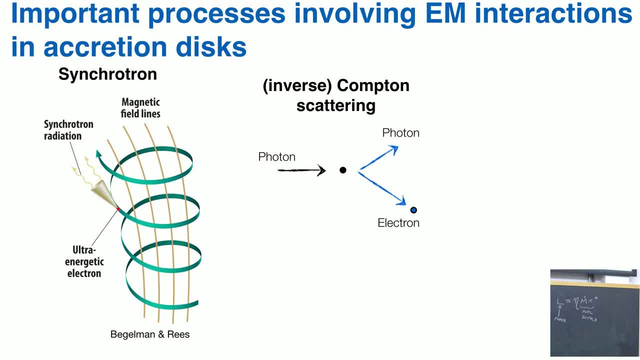 field, if you wish, And they will scatter each other, Depending on who gets the more energy. you call it complex scattering or it's quantum scattering. The other process is that electrons will interact through Coulomb collisions with protons And they will be accelerated. 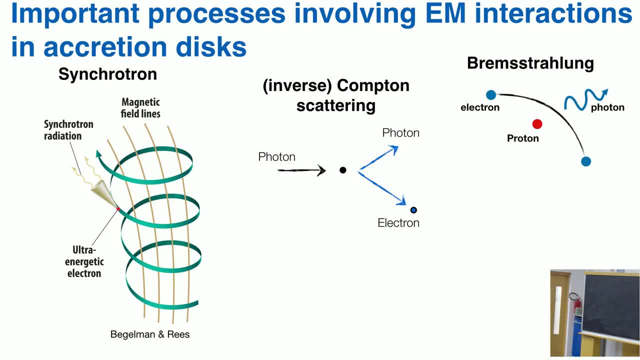 They are lighter than protons. They will be bent, Their paths will be bent And they will emit radiation. This is what we call And, finally, this is important for it. So these three processes here they release what we call continuing emission. 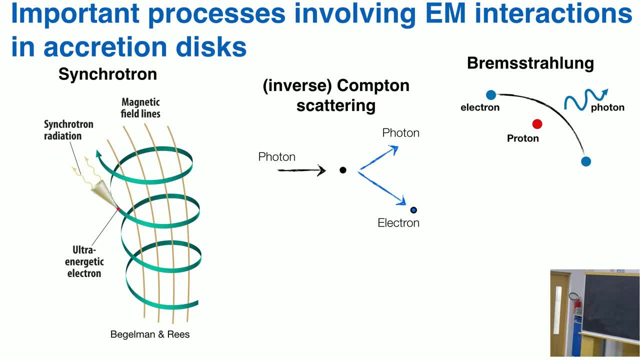 Because if you look at the electromagnet, if you look at the spectrum and you work out the equations, it's a very smooth, broad spectrum characteristic of these interactions. This by itself is a whole course on radiation theory. It's a six-month course that we teach. 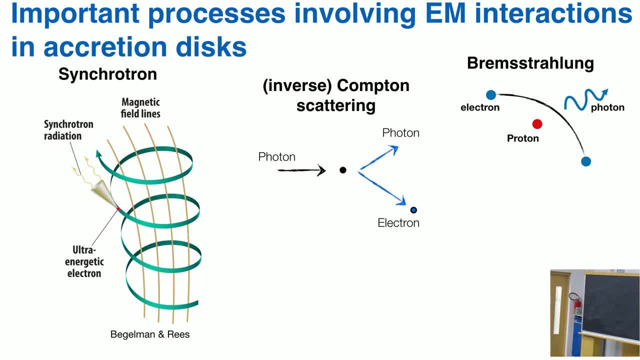 to our graduate students in our astronomy institute. There is a further process which is important, which is ionization. In other words, if you throw a charged particle into an atom or you throw a high energy photon, you can remove electrons from the atom. 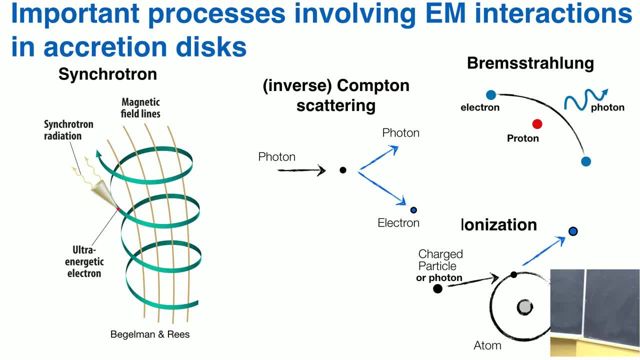 So this is ionization. of course. The thing is, when the electron recombines with the nucleus, you will have emission lines released because of this recombination. I will talk a little bit more about emission lines, Because this is a theoretical physics institute. 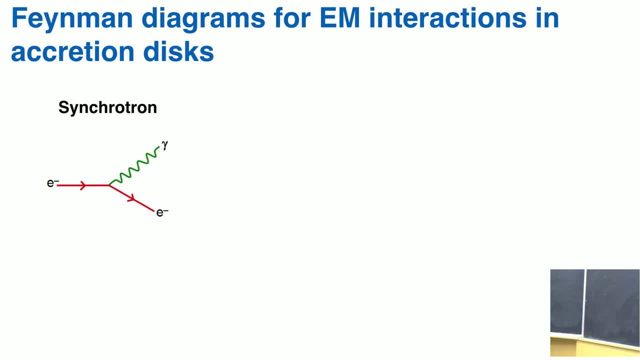 I am obliged, contractually obliged, to show Feynman diagrams. So these are the Feynman diagrams. These are the diagrams of the electromagnetic interactions. This is the synchrotron Feynman diagram. This is the inverse Compton-Feynman diagram. 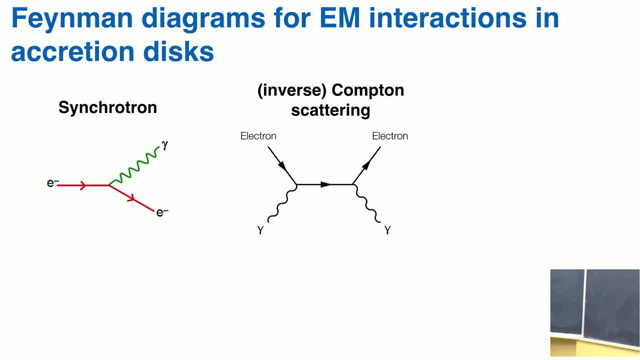 If you wish, time is horizontal and space is vertical. here This is the Feynman diagram for the Brant-Stralon interaction. And finally, I will not show a Feynman diagram here, but I just wanted to say the line emission is important. 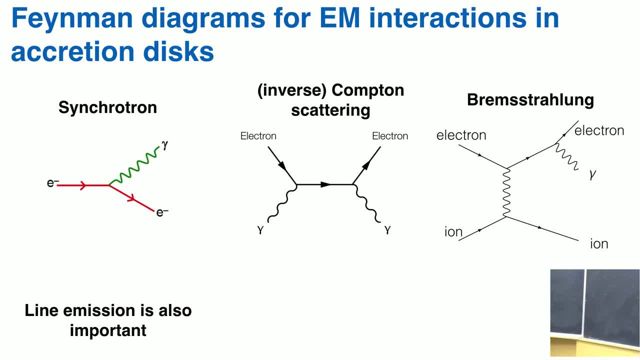 because you have ionized gas which the nuclei recombine with electrons. As the electrons recombine with the nucleus, they like to go back to the ground state And as they transition down to lower energy levels, they release emission lines which are really telling us. 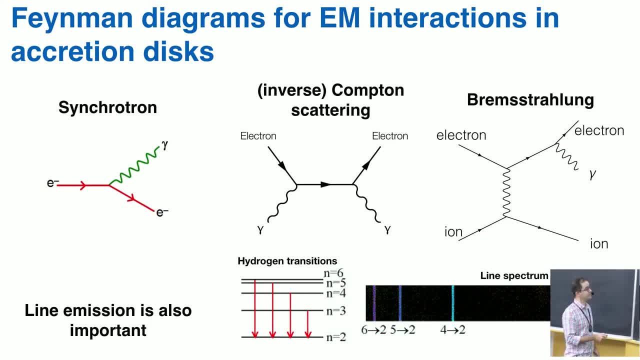 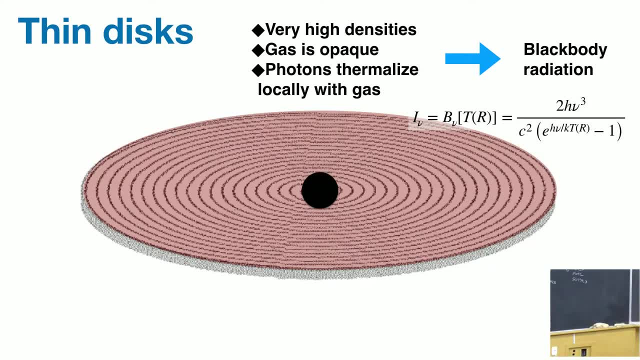 that these gases, they obey the quantum mechanics. okay, quantum transitions. So let's begin talking about the continuum processes. Let's look at the field. So this is a thin-disk solution with very high accretion rates. So these thin accretion disks, they have very high densities. 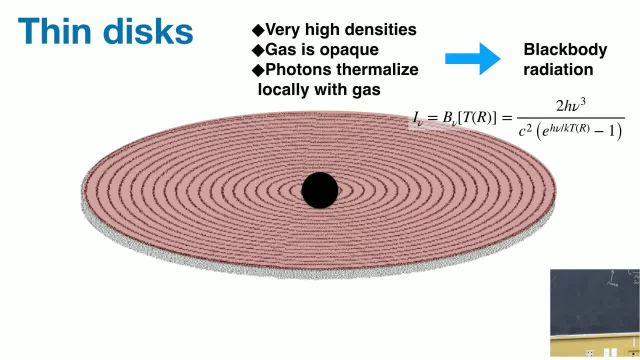 The gas is basically opaque. So, in other words, the photons will have a lot of time to interact with the protons- sorry, with the electrons and the gas- And they will essentially reach an equilibrium where the photons and the electrons will be described by the same statistical distributions. 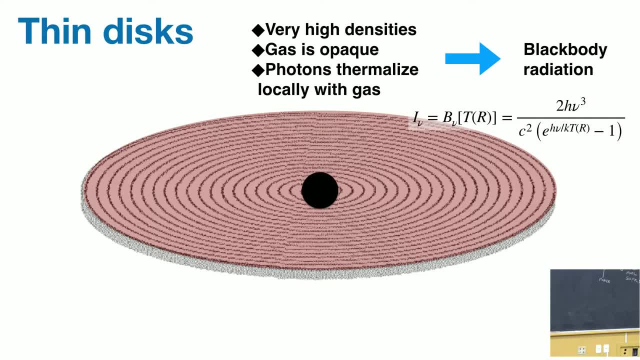 with the same temperatures. okay, So when you have the photon fields in equilibrium with the electron field, you have black body radiation where both are described by the same temperature. So at each radius of this accretion disk it is locally emitting with the Planckian spectrum. 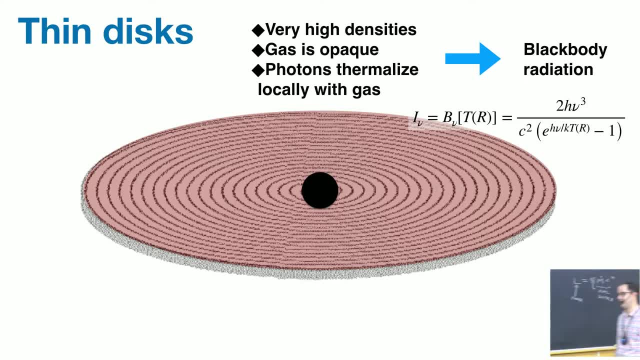 the black body. So if there are thin disks in nature, we expect to look with a telescope to a black hole. We will not see Hawking radiation. Okay, Sorry if you are excited about Hawking radiation, but we will not see Hawking radiation. 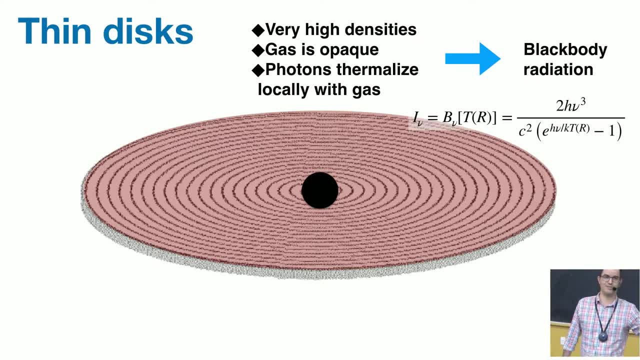 We will probably not see extra crazy dimensions- Okay. We will see the four dimensions of spacetime, something emitting in four dimensions- Okay, And we will expect to see something that emits like a black body. The black body radiation comes from the gas. 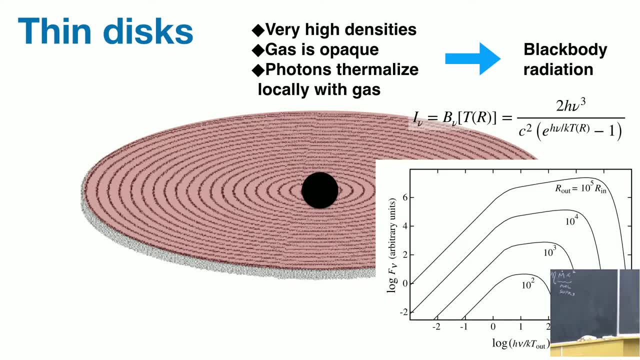 around the black hole. This is the characteristic spectrum of black body radiation, So it has this characteristic shape. As Planck taught us and other people taught us over the last century, it has this characteristic shape. This is the frequency of radiation. 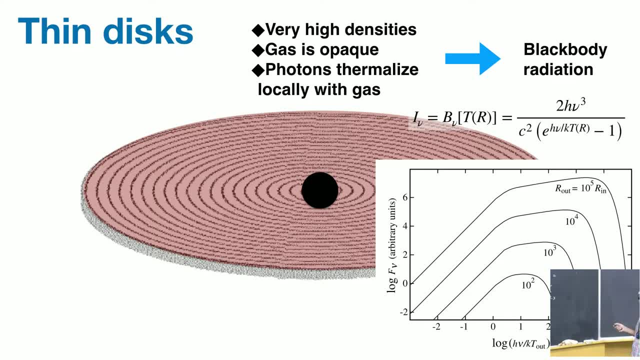 This is the intensity of radiation in logarithmic scale, And it has this shape of a peak, And the peak drifts towards higher energies as you increase the effective temperature of your gas. Okay, In this case, yeah, this is the basic picture of a black body radiation. 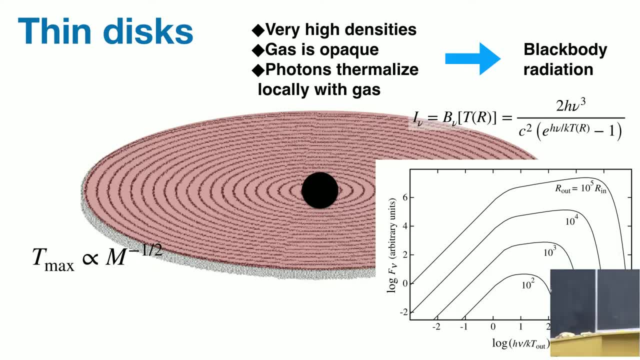 So if you work out with the equations for the black body physics, you will find out that the maximum temperature of the black body is inversely proportional to the mass of the central object. So for fin accretion disks around supermassive black holes, black holes with masses of millions or more. 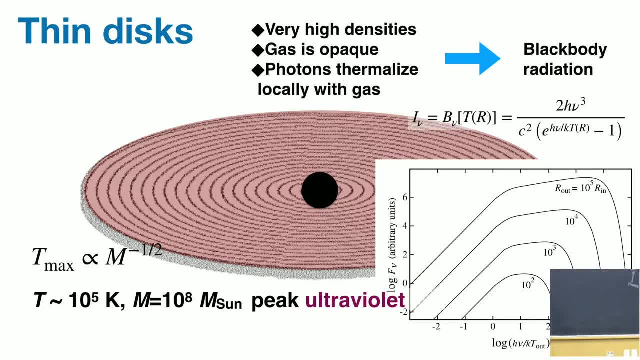 than millions of solar masses collapsed inside the horizon. we expect the temperature to drop. We expect the temperature of the gas to be the maximum temperature to be around 100,000 Kelvin. Due to the physics of black body radiation, we expect the peak of the electromagnetic emission. 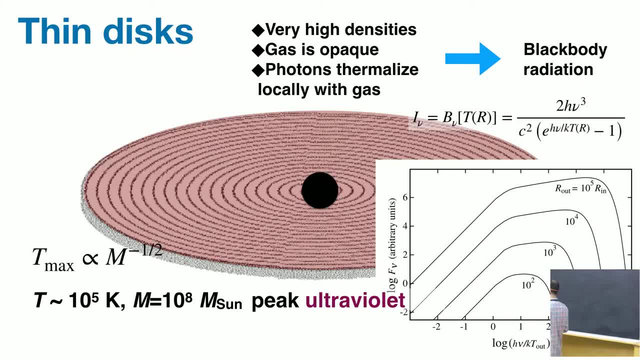 to be in the ultraviolet. So if you want to see the signature of the presence of supermassive black holes, you want to find a telescope sensitive in the optical to catch the lower end of the black body emission and ultraviolet. Okay, 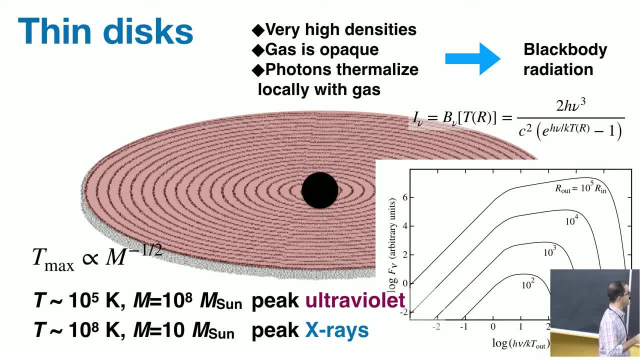 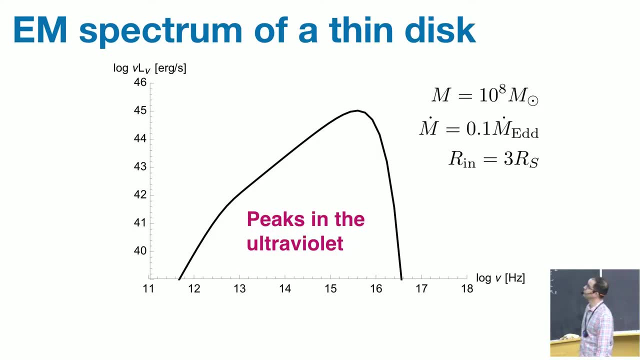 On the other hand, if you have stellar mass black holes with masses of 10 solar masses- comparable to the 10 solar masses- the temperature will be almost 1 billion degrees and you expect the peak of emission to be in x-rays. So you need x-ray telescopes. 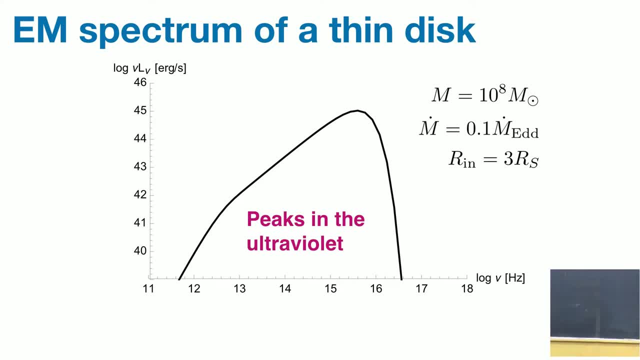 This is a simple calculation I did with the physics of black body, showing you the spectrum logarithm of frequency in hertz versus logarithm of luminosity. This is the typical black hole in the center of a galaxy, with a lot of gas being provided to the black hole. 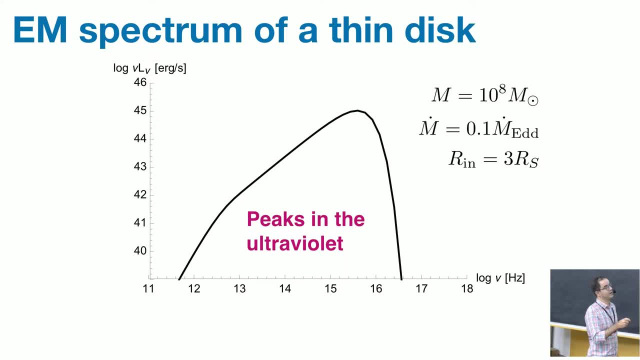 and it peaks in the ultraviolet. Okay, So if you are close to this accretion disk, you will get a lot of sunburns. Okay, You will get probably skin cancer. if you go close to this black hole Peaks in the ultraviolet. 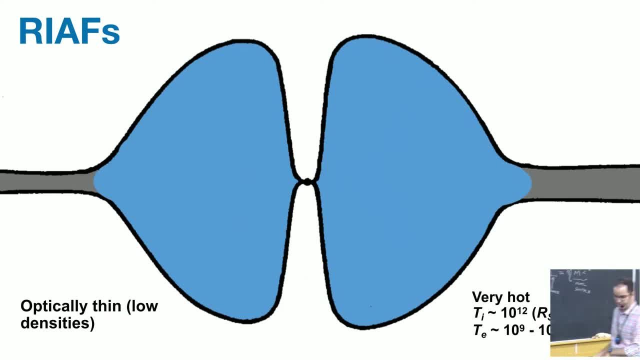 The other main solution that I discussed in this course. I have really to take care of the time here. I didn't. What time am I supposed to finish my lecture? Are you guys keeping? I was not really paying attention. Starts at 2.30.. 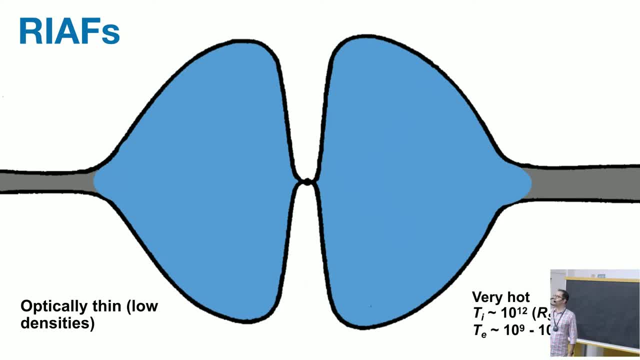 Should end at around 3.15.. No, sorry, Around 4.00, 3.45, 4.00.. Okay, 3.45, 4.00.. Let me put a timer here. Very good. 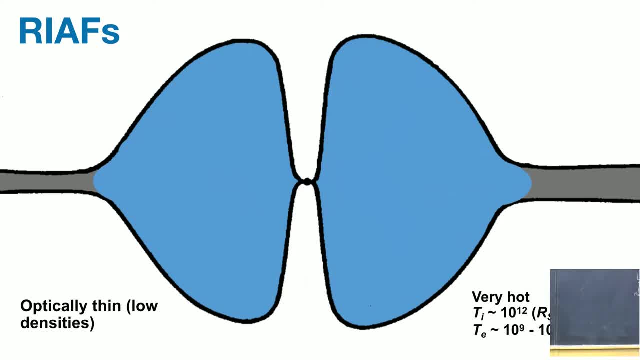 So the second time of black hole disk solution that we discussed is the so-called RAIA, radiatively inefficient accretion flows. So the RAIA: it inflates like a balloon vertically because of the high thermal pressure, because it doesn't like to radiate the heat generated. 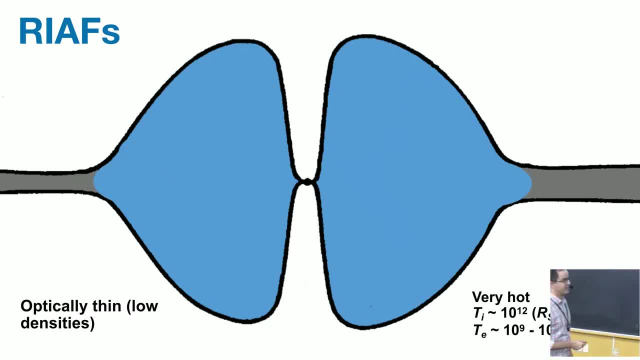 locally as radiation, So it inflates like a balloon, a heated balloon. So RAIAs, because they have densities, they are what we call in astronomy optic, In other words, they are transparent to most radiation. So if there is a photon generated, 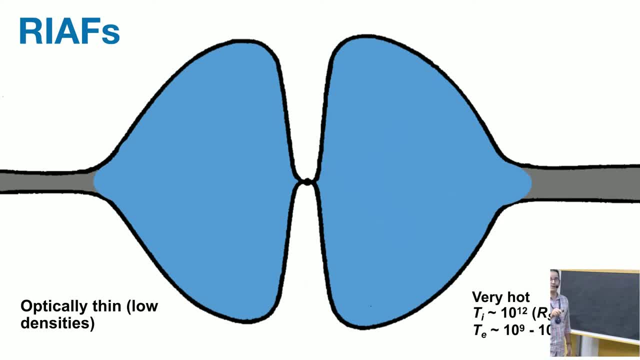 inside the heart of the ray of. but if a photon is generated around here, it will easily, because it doesn't really interact with the gas- That's what we call optically thin in astronomy- And because another interesting thing is that ray ofs they get extremely hot. They get extremely hot. By hot I mean they develop what we call two temperature plasmas, where there is a stratification of the temperature of protons and electrons. The electrons: they reach temperatures going up to almost 1 trillion Kelvin. 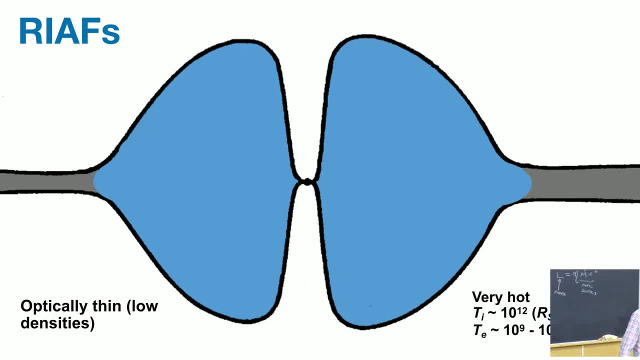 This is a huge temperature, close to what we call the virial temperature of the system. So a couple of interesting processes. radiation processes start getting important in a ray of at such high temperatures and at low densities. The first radiation process is that we 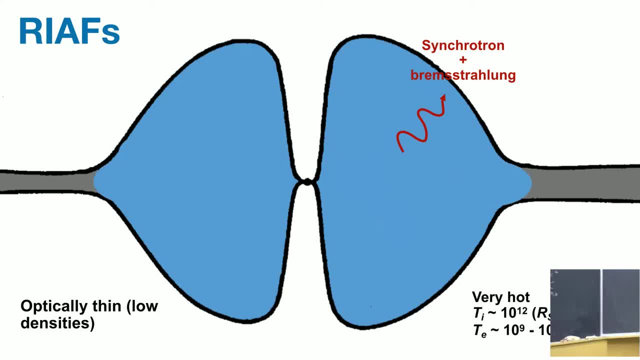 expect reasonably strong magnetic fields, turbulent magnetic fields. So we expect reasonable amounts of synchrotron and Brønstrøm radiation: synchrotron because of the magnetic fields, Brønstrøm because of the protons and the electrons. 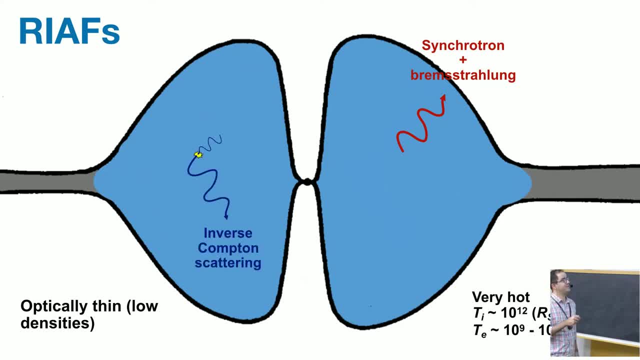 And we also expect the photons to interact with the electrons, The electrons in the disk. so we expect normal Compton scattering, but the inverse Compton scattering, where the relativistic electrons will actually give energy to the photons, Usually in laboratories here on Earth. 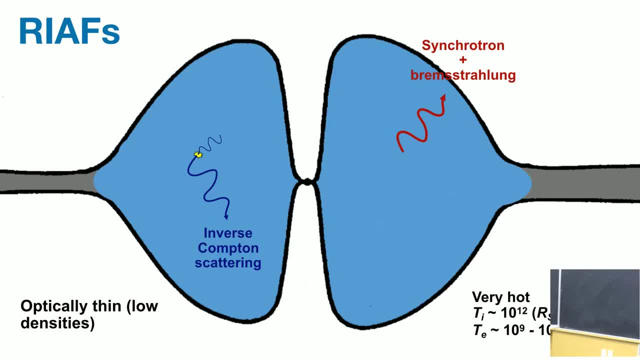 we see normal Compton scattering, But in this plasma there is inverse Compton scattering. Oh, and also we expect there are some traces of a thin disk outside the ray of, but this is one of the weak. this is one of the puzzles in accretion disk theory. 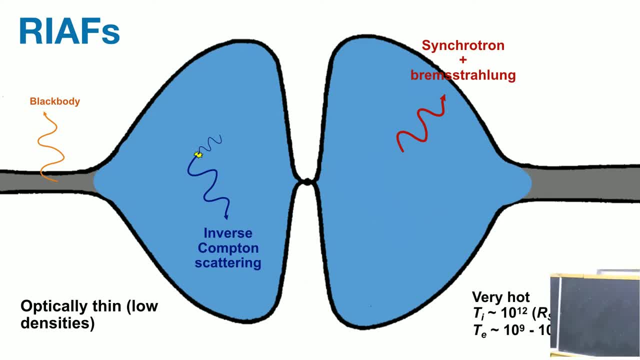 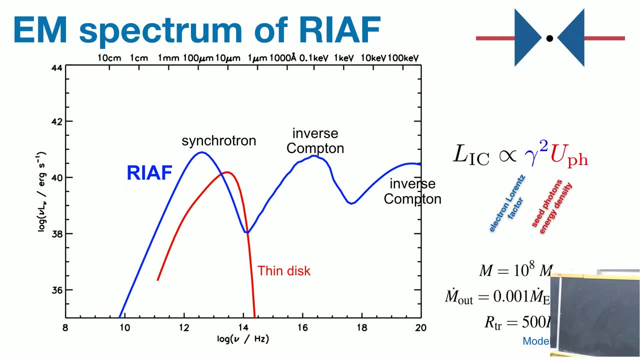 to understand this transition, this border of the ray of. We don't really have a theory for this dramatic thermodynamic transition between the two solutions. It's one of the outstanding problems in accretion disk theory. So the spectrum that you expect from a ray of. 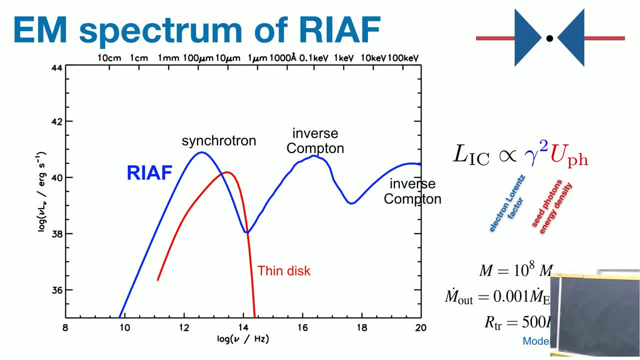 is way more complicated than the spectrum from a thin accretion disk. There's an x-axis, this logarithm of the electromagnetic field. This is the electromagnetic frequency, Here is the luminosity, And you expect to see a way more complicated spectrum. 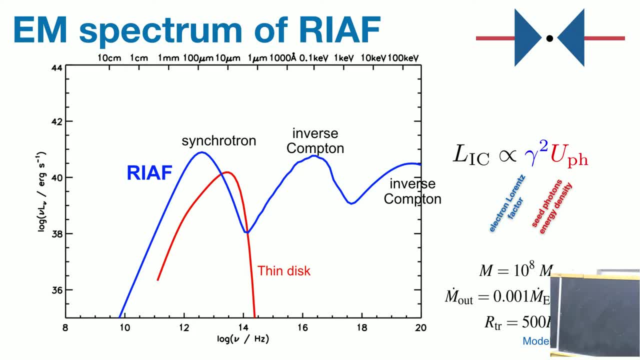 with a synchrotron peak in the radio, an inverse Compton peak in the x-rays and further peaks of the inverse Compton emission which are related to the electron Lorentz, the micro-physical Lorentz factor of your electrons. 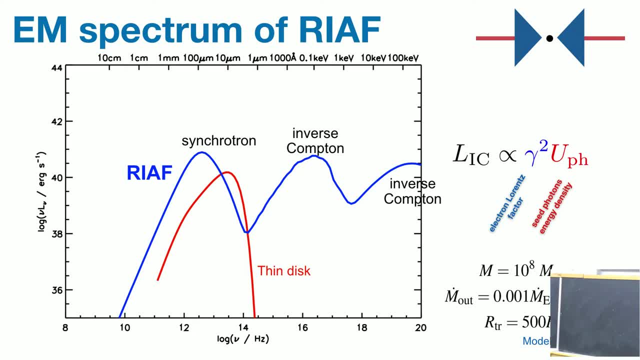 and also the energy density in your radiation field. This is how you can work out this expression: by working out the radiation theory. here I computed this spectrum from a model that my group has. We know how to connect the gravity with the plasma around the accretion disk. 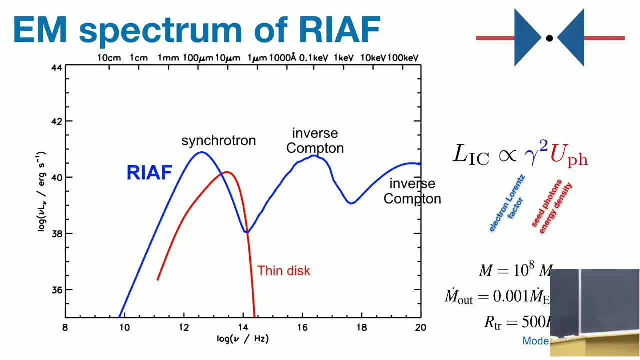 And so we can more or less easily. if you have questions, you can ask my student, Ivan, who is sitting there. He's an expert in computing this kind of spectrum And he can describe you the paper he published a couple of months ago. 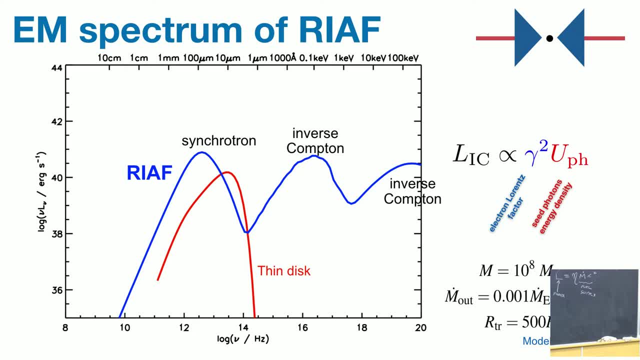 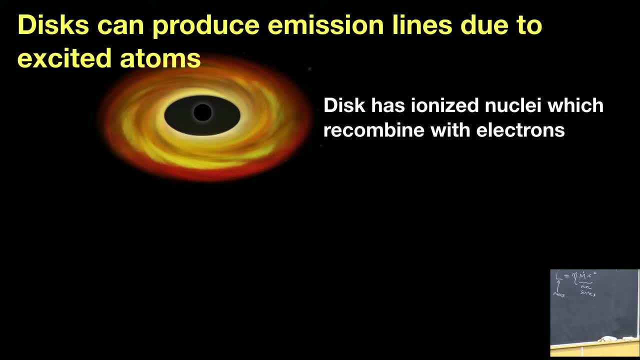 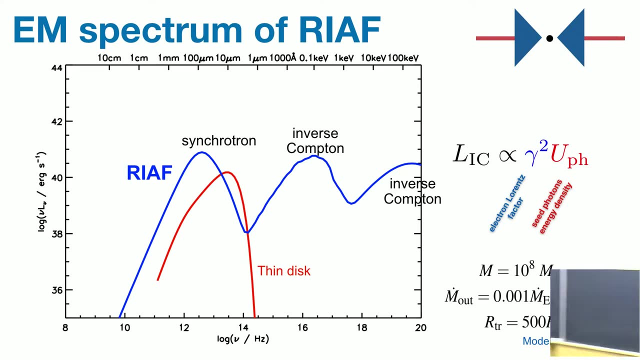 Where he played. I hope he had fun playing with these models. Did you have fun, Ivan? Okay, Right, There is literally decades of work behind the work, decades of work behind these plots that I'm showing you here, So I am simplifying this in an incredible way, okay, 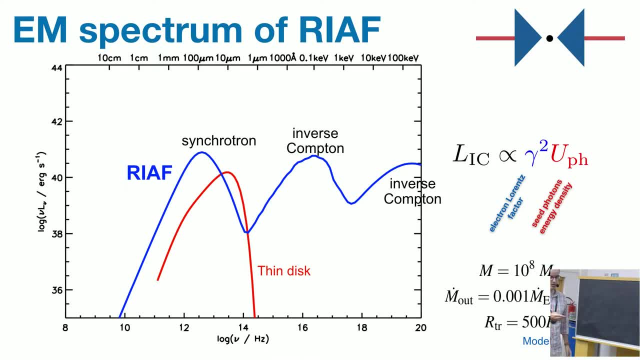 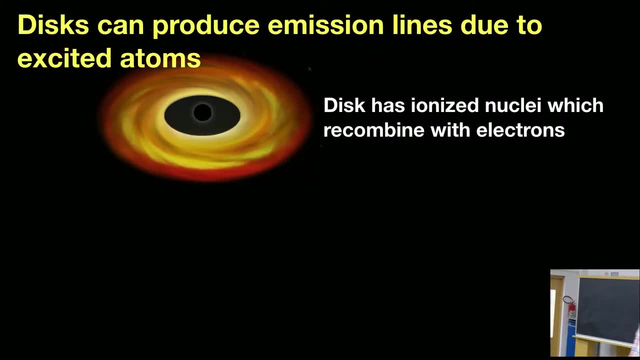 There are a lot of math, a lot of physics in what I'm showing you, But my time is limited So I have to move on. And now let's talk about not continuing electromagnetic radiation, but direct delta kind of electromagnetic radiation in the form of emission lines due to quantum. 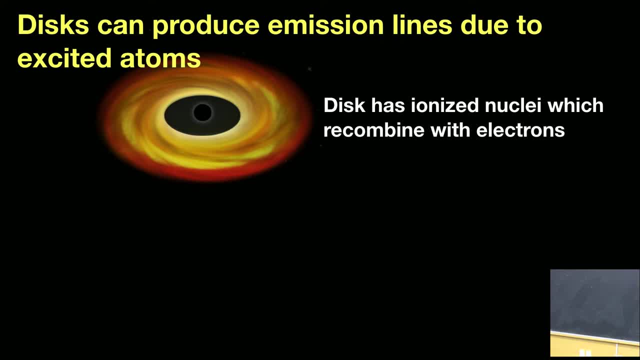 electron, quantum transitions, energy transitions, So the disks around the black holes. they can also produce these emission lines because the heat energy can ionize the atoms. Then you have free electrons And then the free electrons, they can ionize the atoms. 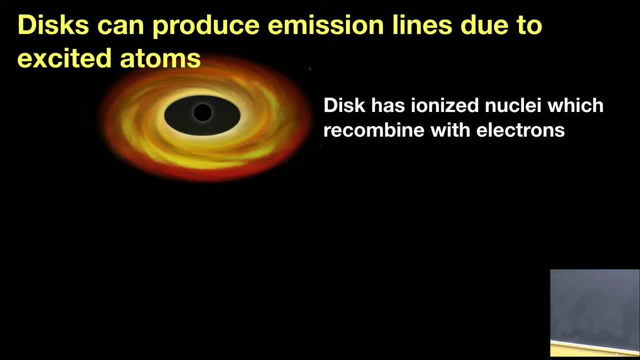 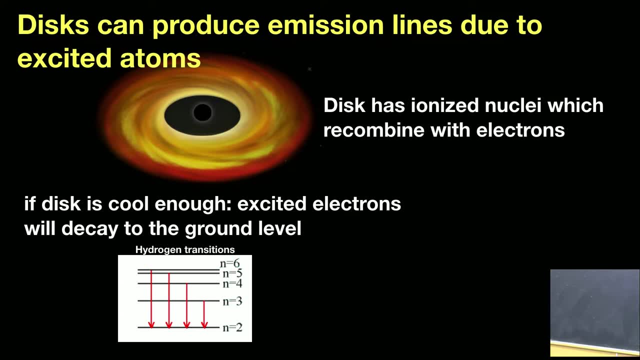 Then the free electrons. they can recombine with the nuclei And then by, as I mentioned, by going back to the ground level state. every time the electron goes down in the energy level, it releases an emission line, And so you expect to see emission lines being released. 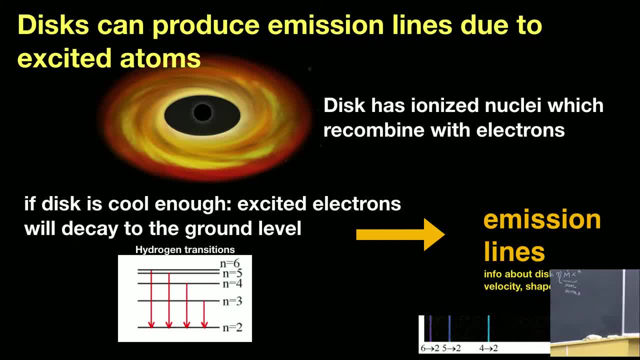 by the surface of accretion disks due to these transitions, these kind of transitions, electron energy transitions- And the emission lines you can see. you can see which, if there was no motion in the gas and there was no turbulence, the emission lines would be direct deltas. 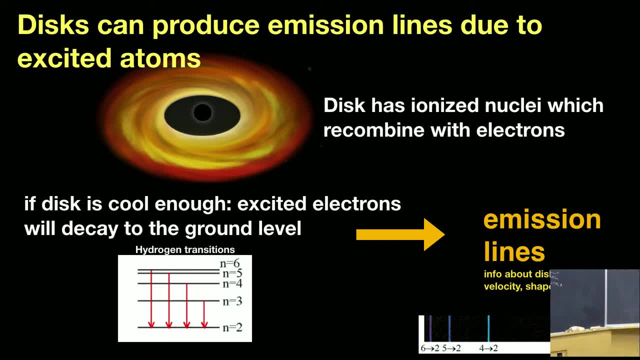 precisely located at the energy of the electron energy transition. However, we don't have stationary, we have relativistic gas, And so we hope that by looking at these emission lines, we can learn something about the way nature likes to feed astrophysical black holes. 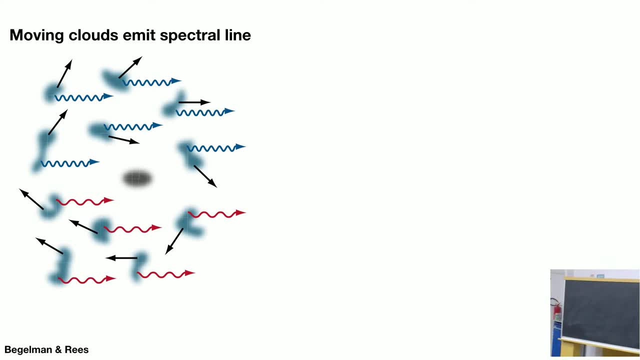 So the idea here behind the physics of emission lines is somewhat simple. The idea: imagine that you have moving clouds which are each little moving cloud is emitting some spectral line. Imagine there are electrons in each of these clouds. going down from the level three to the level two, let's say: 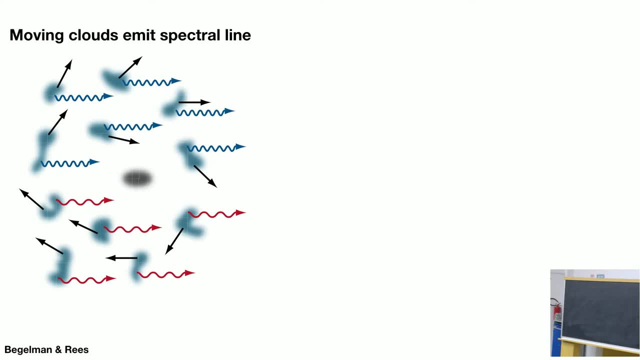 Imagine this is hydrogen, only hydrogen. And imagine now that in the moving frame you will see a direct deltas, A direct delta located at the energy of the transition. The problem is: imagine you have clouds which are moving around the central object. 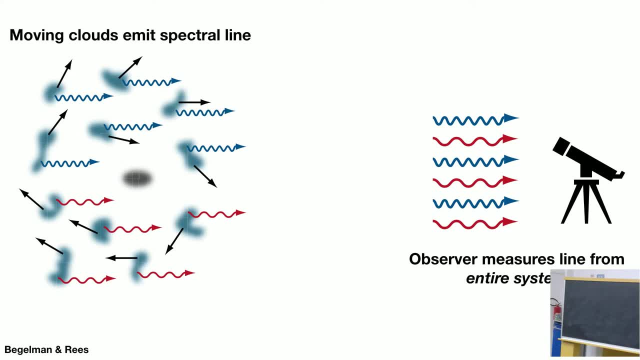 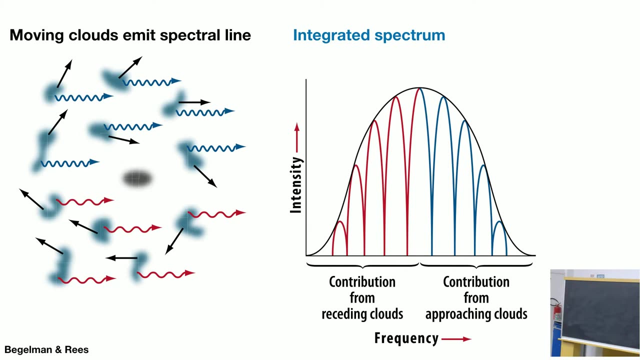 And what you are detecting. you are not resolving the motion, usually of individual clouds. You are detecting all the emission lines together, unresolved from a single point, and you get a collective measured line from the entire system And what you would expect from the emission line is not a direct delta. 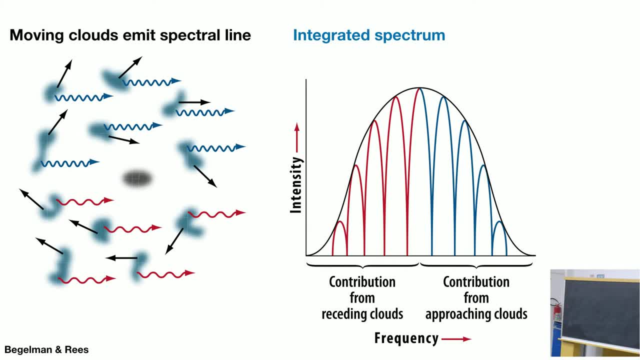 You would expect something much more, a little bit more complicated than a direct delta. You would expect the integrated emission line spectrum to have a contribution of the clouds receding from you. So they are red shifted, so they have lower energies. This is Doppler shifting. this is the physics. 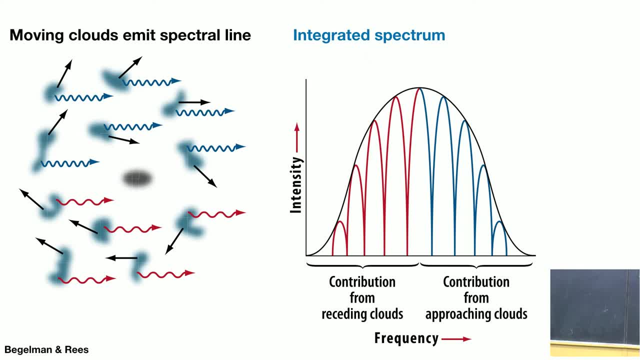 of the Doppler effect applied to the motion, the effect of the motion of the clouds on the emission lines And the clouds which are approaching Towers of the Observer. they, in fact, are moving in the direction of the emission lines And the clouds which are approaching Towers of the Observer. they, 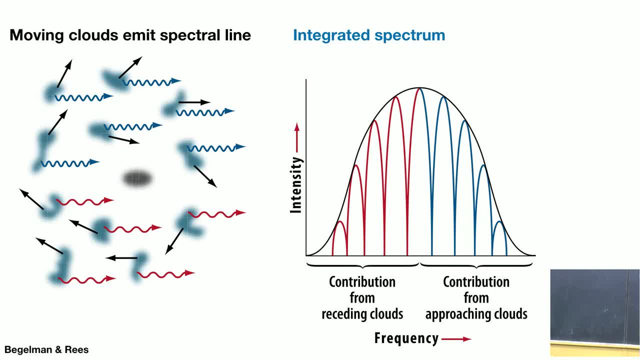 in fact, are moving in the direction of the emission lines, And in this case, the Doppler effect increases the energy. They are blue shifted, And so you expect to see an emission line, in a very simple case, something like this: 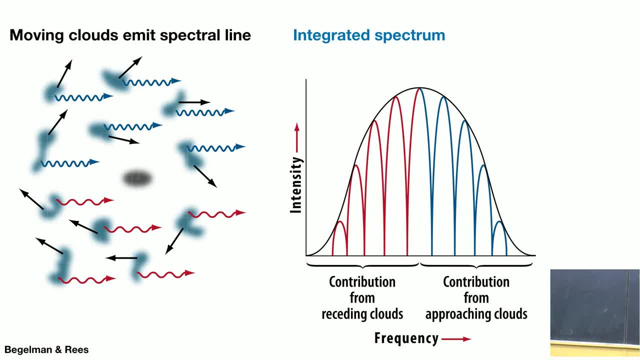 So the Doppler broadening of the line is entirely due to the motion of the gas clouds, So we expect this, so okay. so the width of the line. if you measure the width of the line in the frequency space, you would expect the width of the line to be much larger. 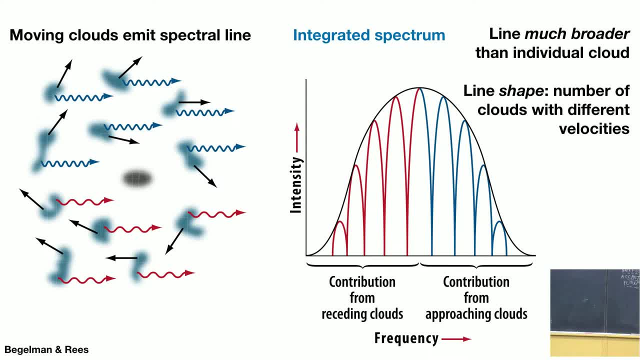 than the individual clouds. It's not a direct delta and you hope, as an astrophysicist, that the shape of the line might inform you about the velocity field of the gas and the shape of the gas and the homogeneities of the gas and perhaps tell you something indirectly about the space. 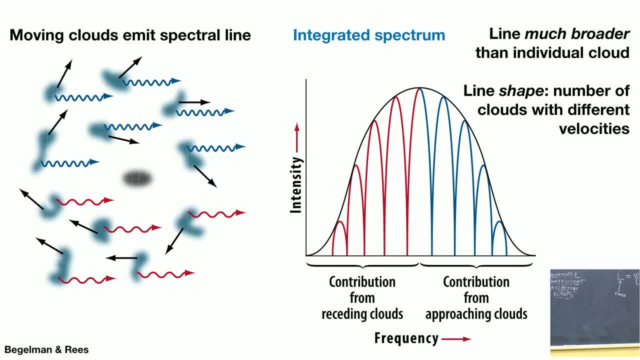 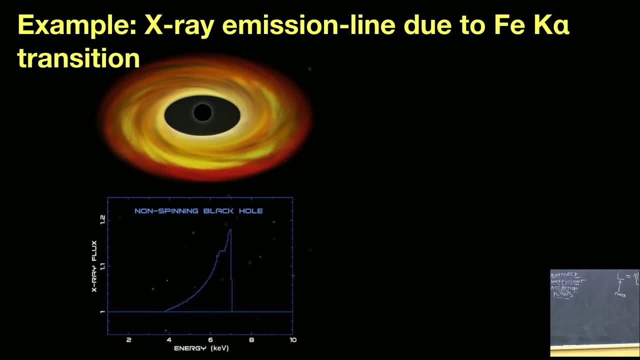 time of the black hole by looking at the emission line. So astronomers have been playing this game for quite some time now. So if you play this game and you model the velocity field of the accretion disk, which is recombining and producing an emission line, and you couple the Kerr metric, this is what 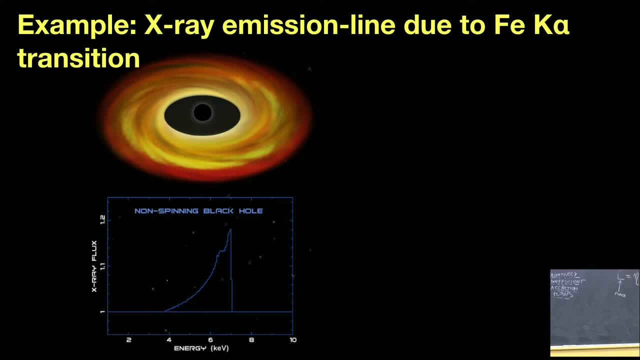 you expect from the iron K-alpha transition. This is not now a hydrogen, This is iron. This is the emission line of electrons decaying going down the energy levels in an iron atom. So this is the model that you expect for the emission line distorted by the gravitational. 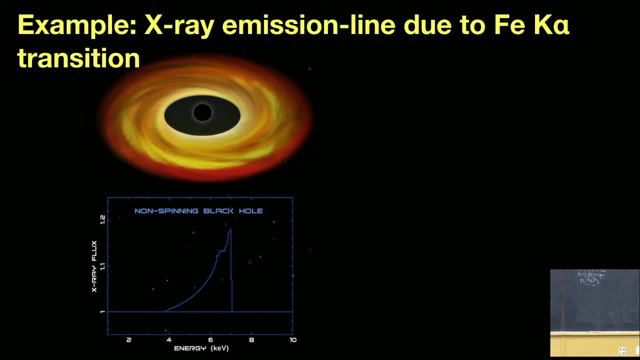 redshift, the usual Doppler shifting around a non-spinning black hole. Remember, this is the ISCO. This is the innermost stable circular orbit around the Schwarzschild black hole, located at 6m. This is, as I mentioned in my second lecture, the ISCO. 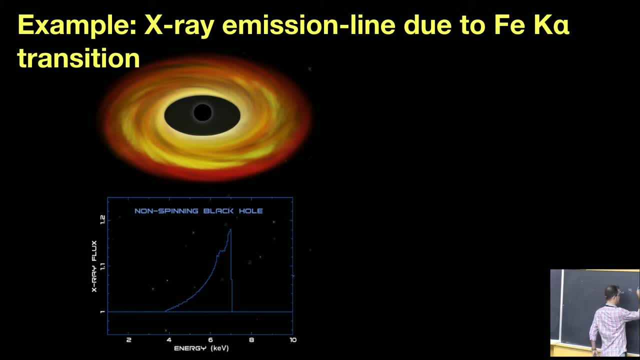 And also, as Ian mentioned in his lecture, the ISCO for a Schwarzschild black hole is located at 6m And also, as Ian mentioned in his lecture, the ISCO for a Schwarzschild black hole is 6m. 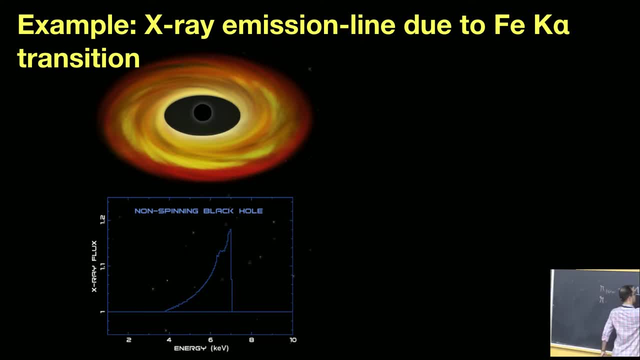 And for a Kerr black hole it can go down. if you have a maximally spinning black hole, it can go down by a factor of 6.. So if you do the calculation, you plug in the space-time, you plug in the physics of. 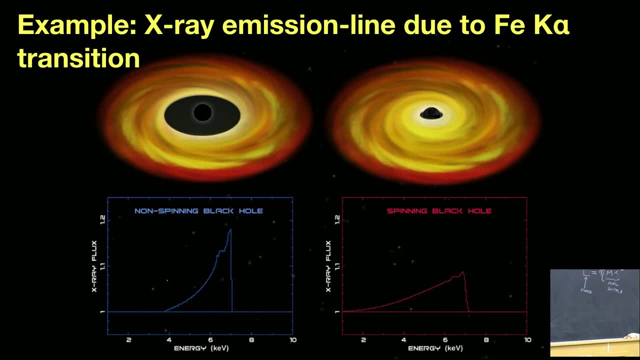 the gas and the physics of the emission line. here is the ISCO. now you have a maximally spinning black, almost maximally spinning black hole black hole And look at the dramatic distortion on the no geodesics of the light that is trying. 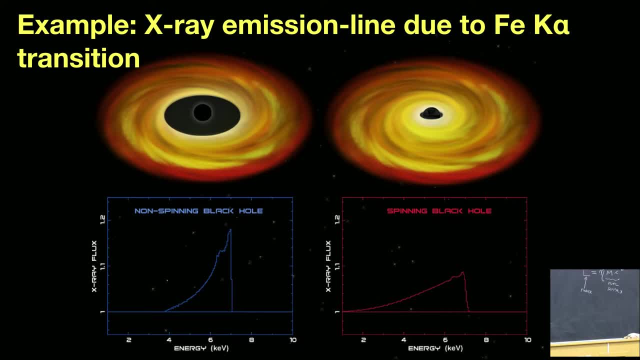 to escape from the accretion disk. You see a dramatic difference in the brightness. You see that the lower energy side of the line extends way down because of gravitational redshift. The line is also less luminous, also because of gravitational redshift. So you expect. 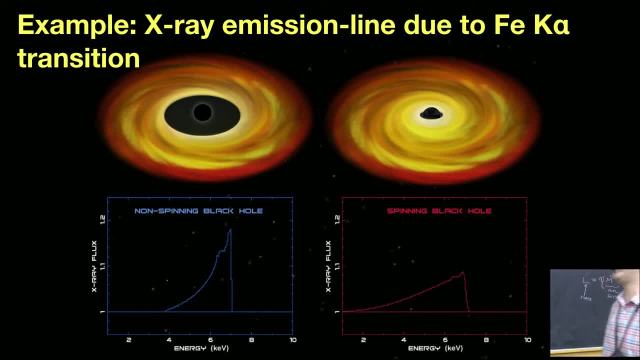 this is amazing. you expect to use electromagnetic observations to probe the spin of the black hole with emission lines. So this became really an industry in the late 90s and the 2000s And still the industry is going now. But it became an industry of trying to constrain the distributions. 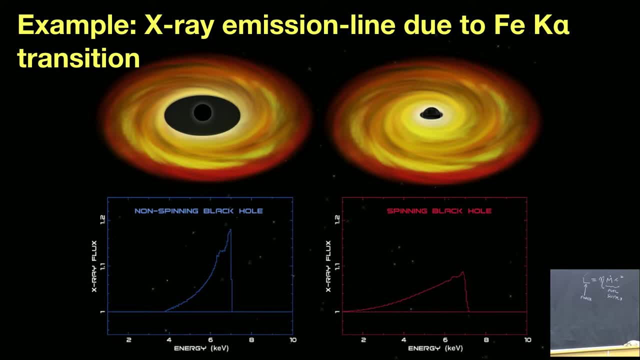 of spins of the curve metric of astrophysical black holes by looking in x-rays to several systems. So this is an industry of trying to constrain the distributions of spins of the curve metric of astrophysical black holes by looking in x-rays to several systems. So this is an industry of trying to constrain the distributions of spins of the curve metric of astrophysical black holes by looking in x-rays to several systems. So this is an industry of trying to constrain the distributions of spins of the curve metric of astrophysical black holes by looking in x-rays to several systems. 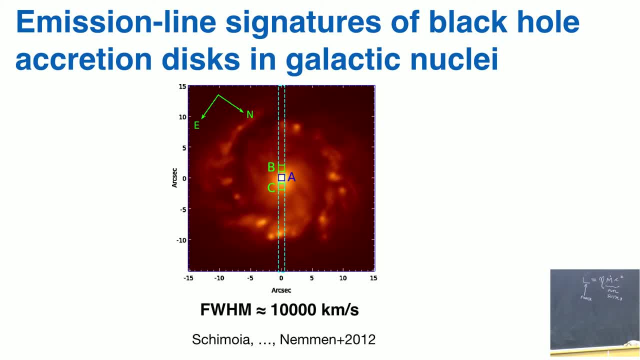 I played a bit of the game myself, but I played in lower energies, So this is a work that we. this was actually, in fact, my first. the work related to this was actually my first paper ever. So we took not x-ray observations, but we took optical observations of the center of a galaxy. 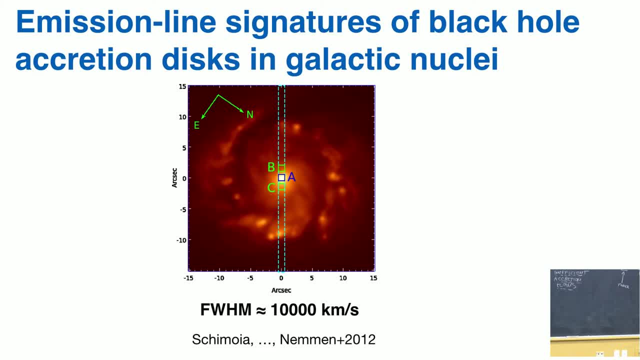 This galaxy is called NGC 1097.. I remember the phone number of the galaxy, So we put what we call a long slate along the nucleus of the galaxy To try to see if we could actually see the emission lines from the effect of the central black hole. 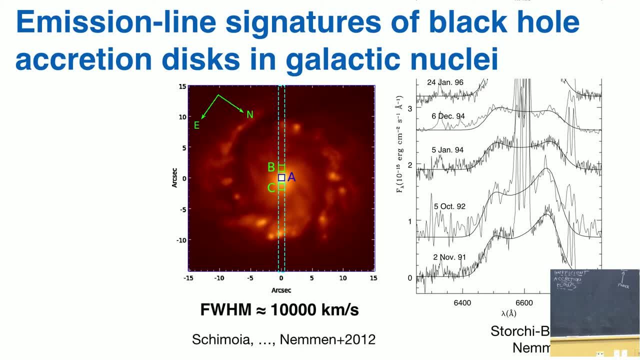 And the emission lines we got here. they were not in x-rays. Actually, the lab frame emission line is what we call hydrogen alpha transition. And look at the sort of beautiful emission lines we saw with an optical telescope. We saw lines which have which are very, in my opinion, strange. 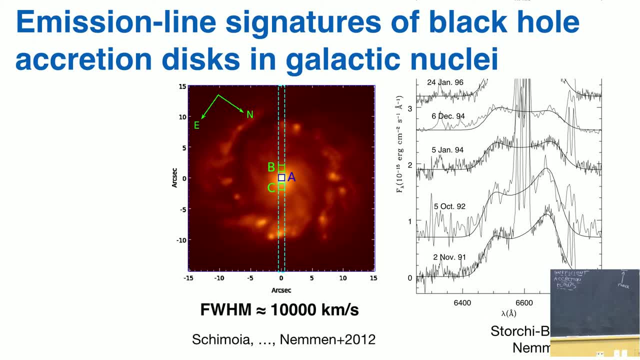 They have this what we call double peaks. They have this emission. Forget about this thing, these direct deltas in the middle. They are not related to the accretion disk of the black hole, And this kind of double peak shape is precisely what we expect when you have an accretion disk. 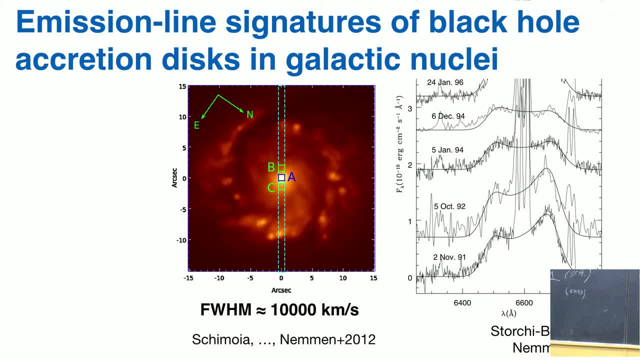 circling around a supermassive black hole. We have a velocity field with typical velocities going up to 10,000 kilometers per second, And we were able to model this emission line and constrain the geometry of the accretion disk around the black hole. 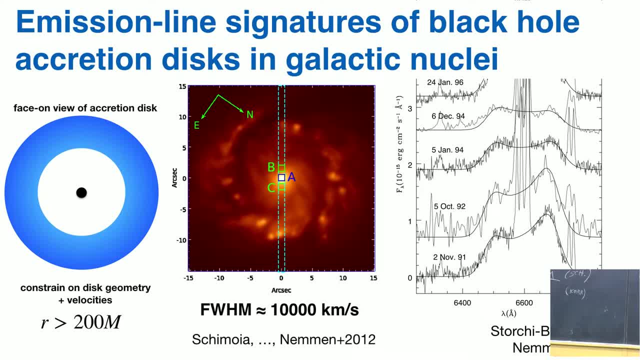 So we constrain that the radius of the accretion disk is above 200 M. So it's a weak field regime of gravity. Okay, so we are not able to constrain black hole spin with this kind of observations, because it's happening almost in the weak field limit. 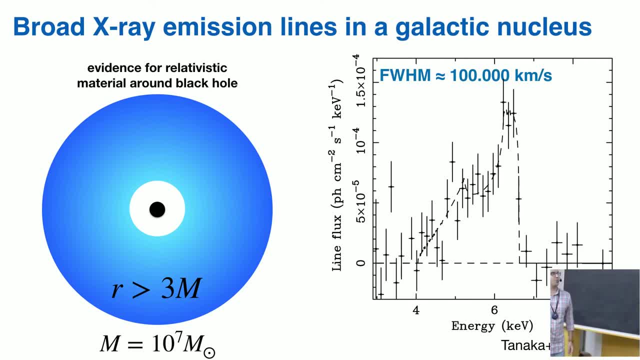 However, in the 90s there was a breakthrough called the, I think, ASCA telescope in the 90s. So they looked at another energy transition in the iron K alpha And they also saw something that looked like the sort of shapes of lines that I presented before. 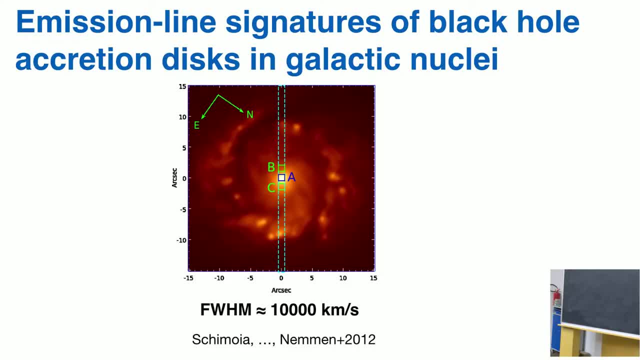 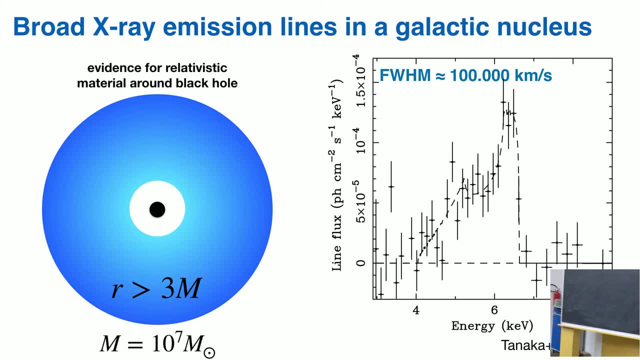 Look at this line and this line- Okay, this is a model. And look at the observation in x-rays. This is fantastic. So the typical velocities here from the Doppler shifting now is relativistic. It goes close to 100,000 kilometers per second. 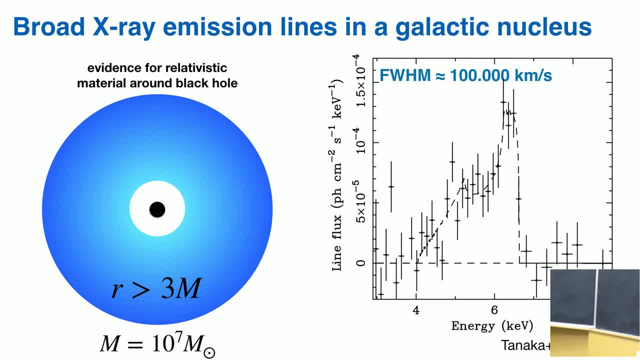 So one-third of the speed of light, And now you are getting very close to the black hole, that radii close to the innermost stable circular orbit, And then things start getting even more fun. So this was a breakthrough, because it was the first direct signature. 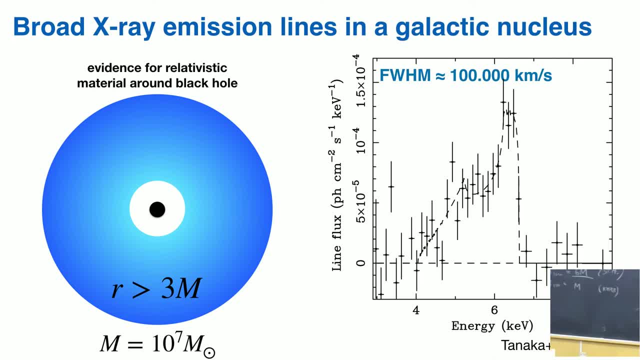 in emission lines of relativistic phenomena in black holes, And the mass of this black hole is around 10 to the 7 solar masses in the center of a galaxy with the name of MC6.. I can make up a number here. It has a strange name, this galaxy. 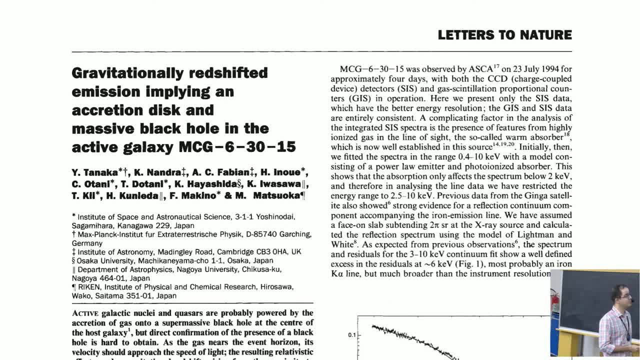 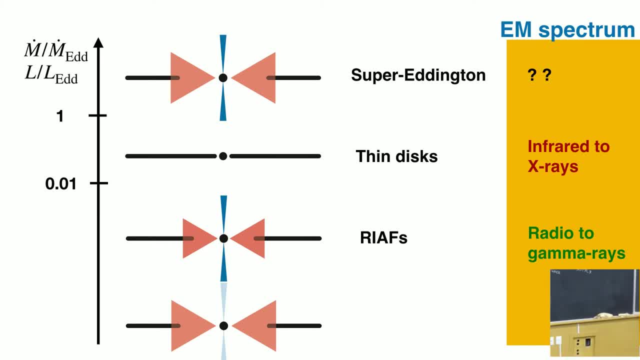 This is the Nature paper of this breakthrough observation. Okay, so this is the basic picture of where you want to look at in the electromagnetic spectrum. if you want to observe the astrophysical footsteps of black holes For thin disks, you should look in infrared, between infrared to x-rays. 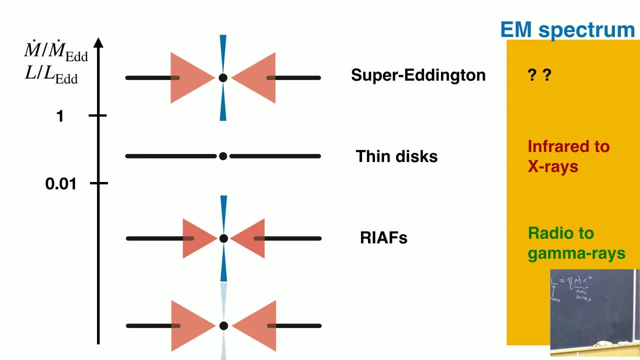 If you have a supermassive black hole, If you have a stellar mass black hole, then x-ray emission. If you want to see the star of black holes, well then you have a broad spectrum between radio to gamma rays. But you have to be very careful about modeling these observations. 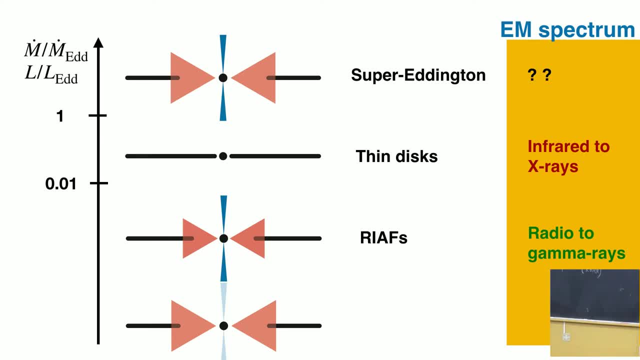 It's not easy to reduce the observations and make it clean enough to leave only the physics of the black hole in the electromagnetic spectrum. okay, When you do astronomy, electromagnetic astronomy, you have to worry about things boring, things like dust emission from the galaxy, stellar emission. 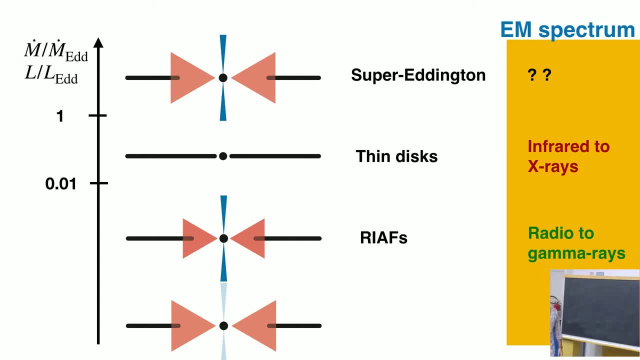 I don't care about stars. Most of my colleagues in the astronomy department don't care about stars, But stars contaminate a lot of these spectra, so we have to remove the stars because I care about the black hole and the black hole physics. 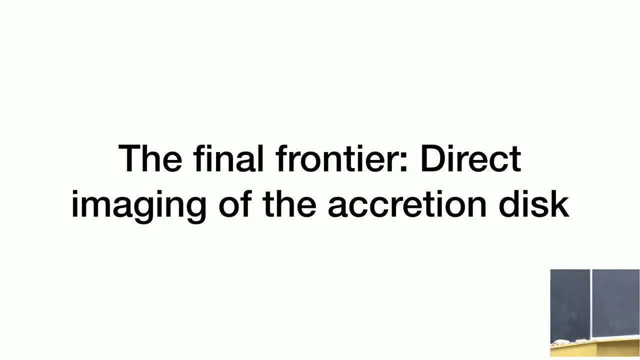 And now we are reaching what I call final frontier. It's really not a final, but you know it's the beginning of a new era in black hole electromagnetic astronomy, of black holes, where we are hoping to have a direct imaging of the accretion disk for the first time in history. 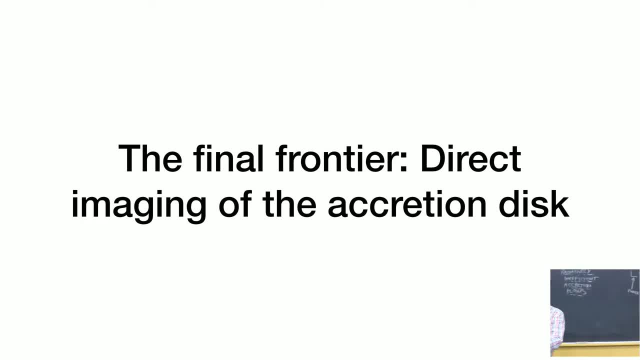 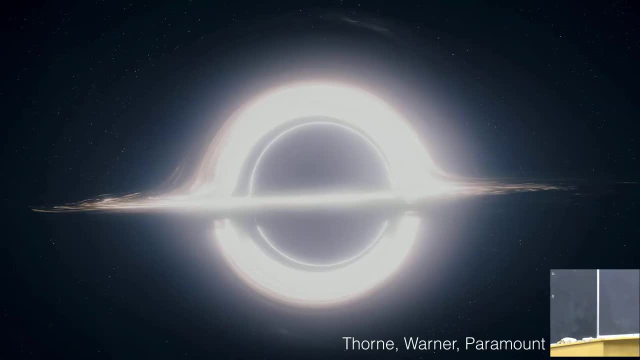 and even perhaps constrain the shadow of the event horizon itself. The goal of this final frontier of direct imaging of a disk around black holes is this: okay, This is what we want to achieve. We want to have a nice, clean image of the disk. 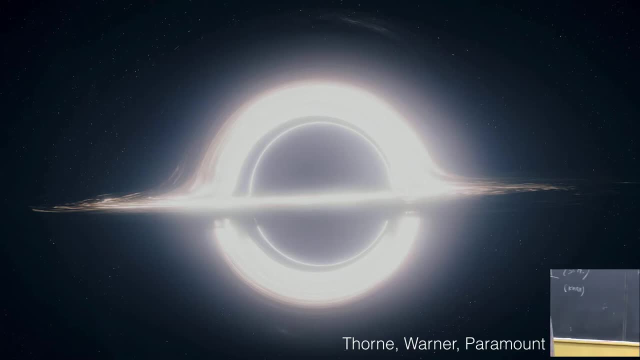 around the heart of darkness and I really make models. You saw me in the Einstein field. Well, for the Kerr metric here we don't expect anything crazy. so it's just the Kerr metric And we want to compare directly our models with the observations. 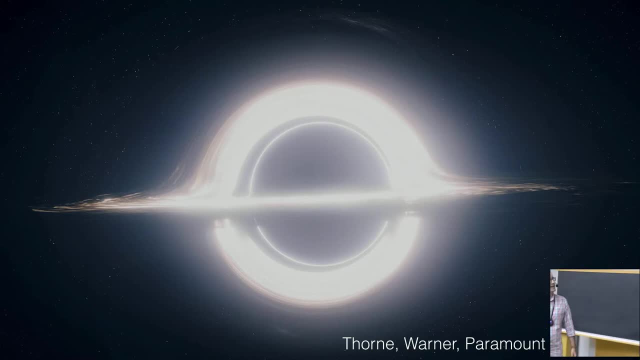 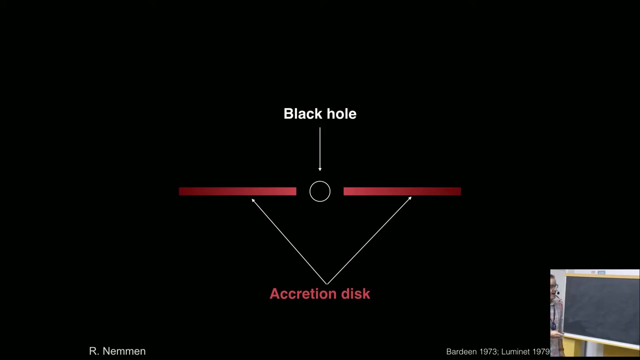 and constrain the spin of the black hole, The thermodynamic properties of the gas, what happens under the extreme curvature conditions to matter near event horizons? This is the ultimate test of Einstein's gravity. So I will not really have time to talk about this. 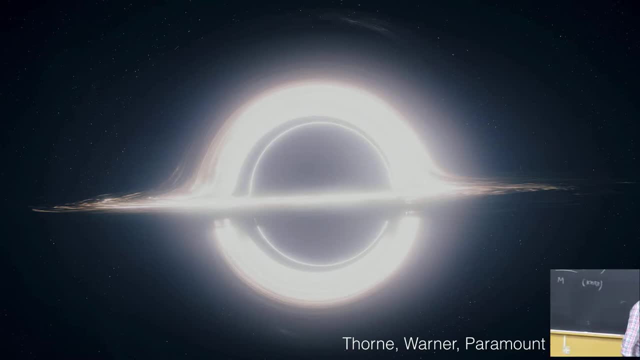 unless I volunteer, if you guys are interested. I know that there is a hands-on session this afternoon, so I volunteer, if there is enough interest, to give you a short presentation about the Event Horizon Telescope, if you are interested, So we can discuss if you want to have some time. 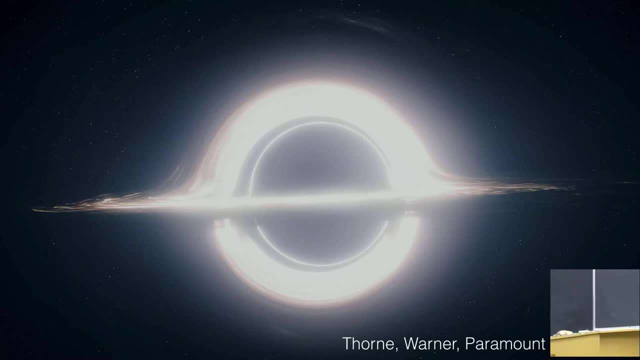 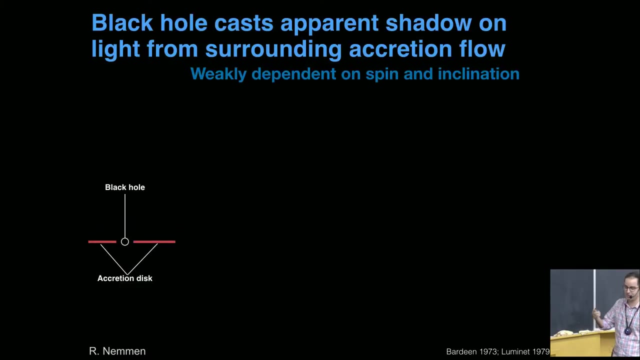 if you want to hear about the Event Horizon Telescope after I finish my talk, okay, So I will not really be able to tell you much now. I have a whole- I gave a colloquium about this, so I have a lot of stuff to show you. 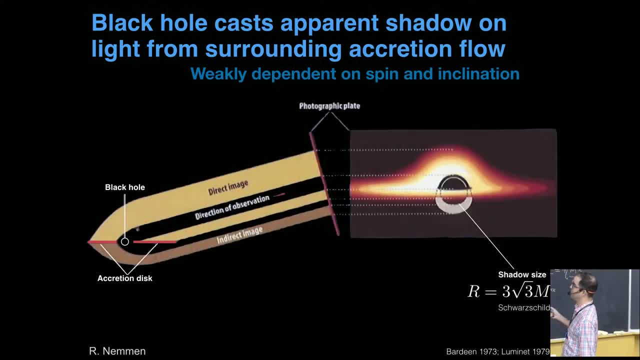 But the idea is you model the knowledge geodesics, tracing the geodesics from the accretion disk and you trace the shadow of the black hole. You make this kind of model. This model is very simple. okay, We have way more advanced models nowadays. 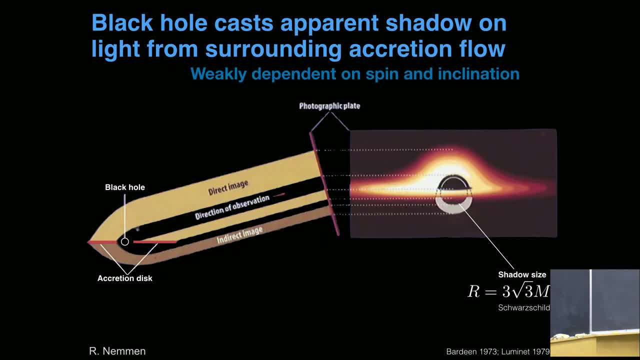 that I describe in my colloquium, And the idea is: by looking at the size, literally the size of a black hole in your image, you can constrain black hole physics and black hole spin. So now let's move on to outflows. 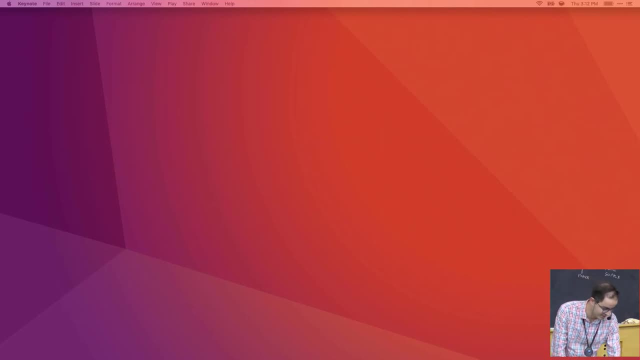 Now we talked about the ends of black holes. Let's talk now about the outflows. Let's talk now about the outs of black holes. Any question about accretion disks, Any question about the ins of black holes before I move on to the outs. 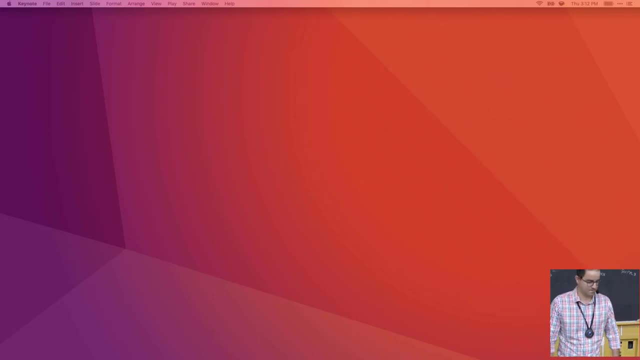 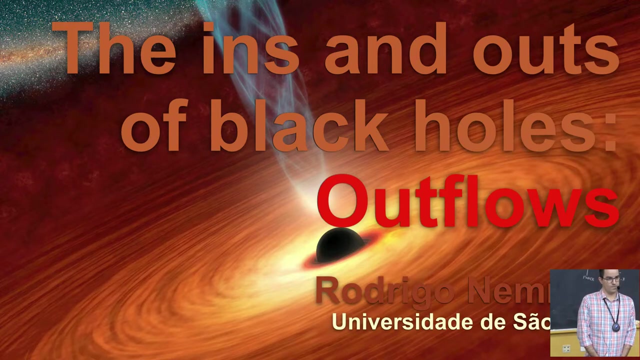 Mm-hmm. Yeah, so he mentioned that you have to take into account the flight escape from the gravitational potential. The gravitational potential, yes. So your question, Yeah, so that's the idea. To build a spectrum, to build a spectrum, the idea. 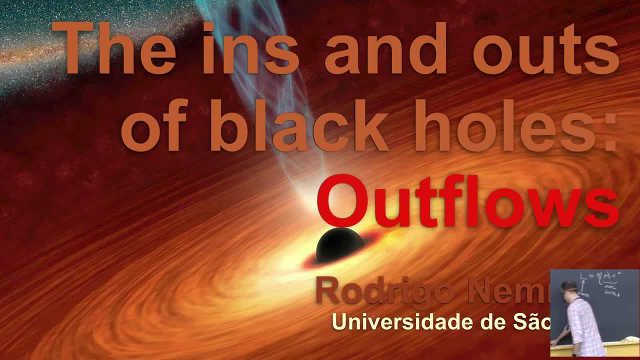 the conceptual idea is simple: You put a black hole, You put the gas distribution on your black hole. In this case, I will just put a blue ray of gas, So you have to generate your photons. So the idea here is that you use the physics of the gas. 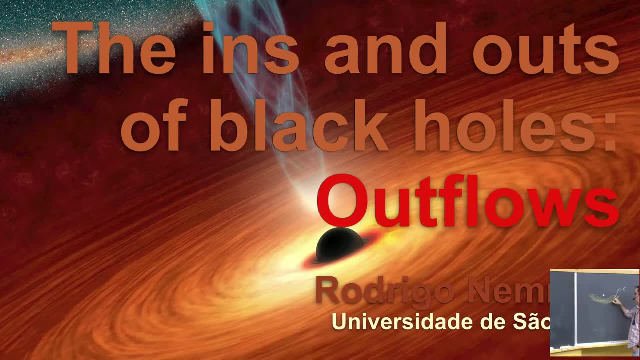 to understand what is the energy of the photon that is being launched at each radius of the accretion disk. So you model this with the wave four vector And the wave four vector, it tells you the zero component, tells you the energy of the photon. 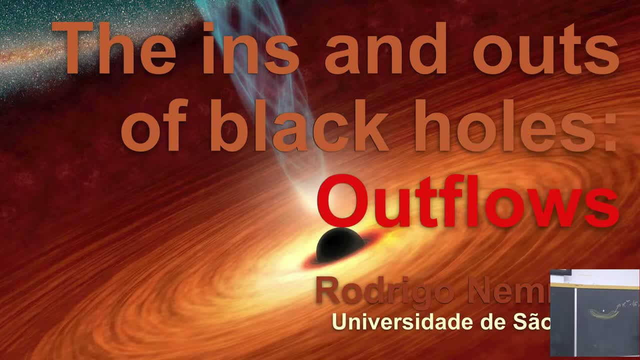 And the spatial components tell you about the wave vector itself. So the wave vector, traditionally in Newtonian physics, the wave vector is pointing at the direction of propagation of the photon And it's normalized such that the modulus of the wave vector is really the frequency of your photon. 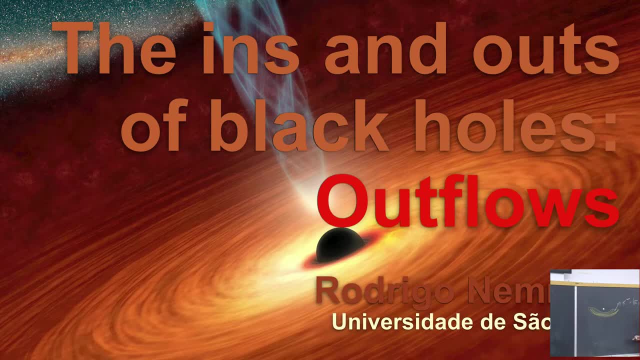 So the idea here is- I can talk more about this in the Event Horizon Telescope talk if you are interested- but the idea is you generate the initial conditions for all the wave four vectors being released by the accretion disk And then you have to propagate these wave vectors. 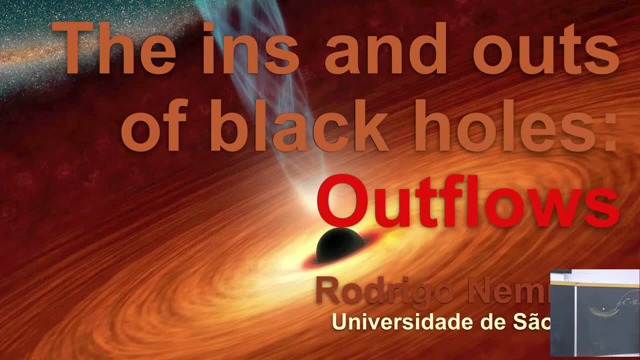 in the space time of the black hole until they reach a virtual observer. And if you collect enough wave vectors, you expect to sample in a complete way the picture of the black hole. And then you expect to compare this cumulative distribution of wave vectors with our ideas about the black hole spin. 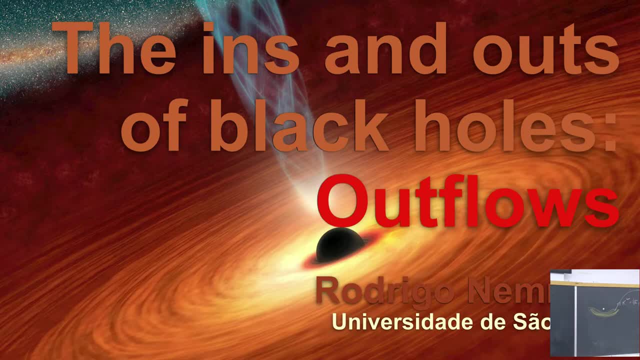 the mass of the black hole, the velocity field of the black hole. So it's an indirect way of using the radiation field to probe the parameters of the space time. And, of course, the way you propagate this is with the geodesic equation. 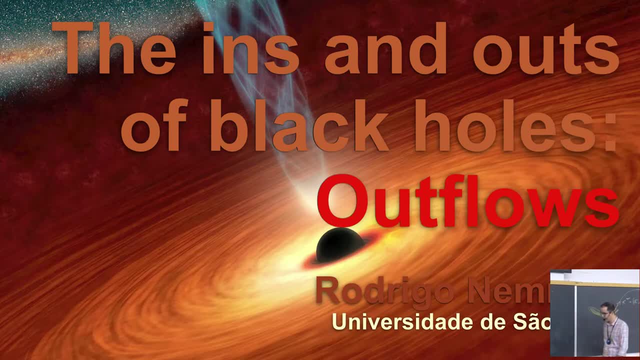 The geodesic equation for no wall lines. There are models. You can do a first model of the system as if it was in thermodynamic equilibrium, but we have strong reasons to believe that parts of the system are out of equilibrium and the physics is way more complicated. 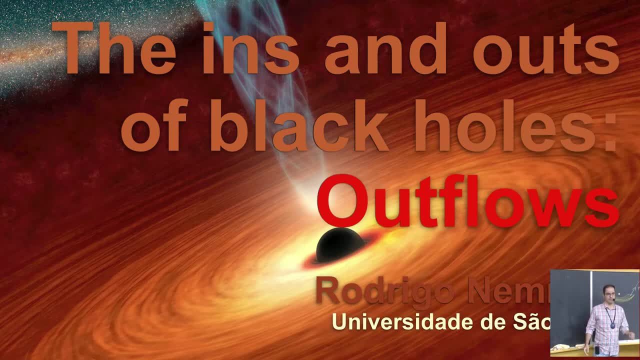 You cannot simply model everything with a black body. It's more complicated than that. We call that non-thermal radiation. So now I will proceed and talk about the outs of black holes. If your black hole is, at a redshift, bigger than 0.1 or 0.1 or bigger than that, yes, 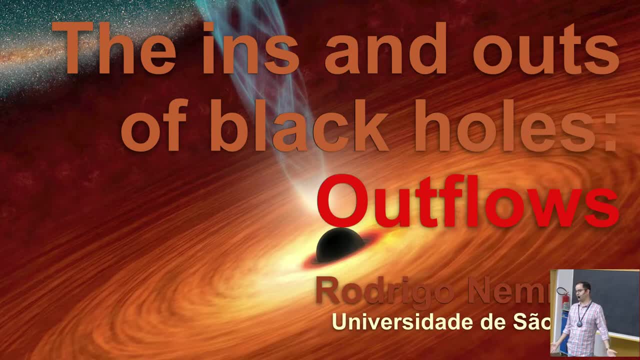 You can use your favorite- I mean the favorite- cosmology is what we observe- the lambda CDM. So then you use the lambda CDM and then you correct the effect of cosmological expansion of the universe on the light that you receive. 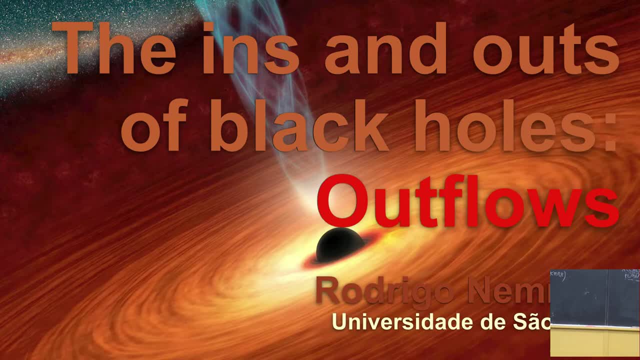 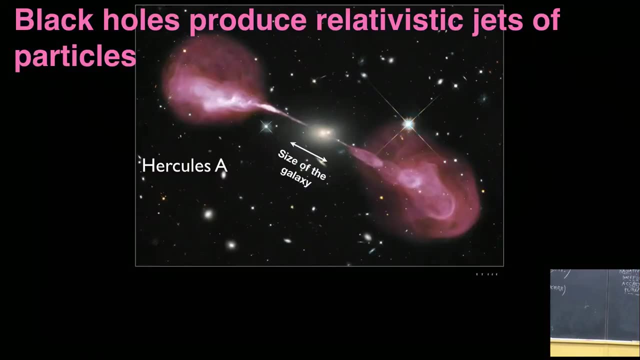 So let's now talk about the outs of black holes, Outflows, Flows that are flowing out of the system, Therefore, outflows. This is a beautiful observation of something that is flowing out of the center of a distant galaxy. We call it radio galaxy, Hercules A. 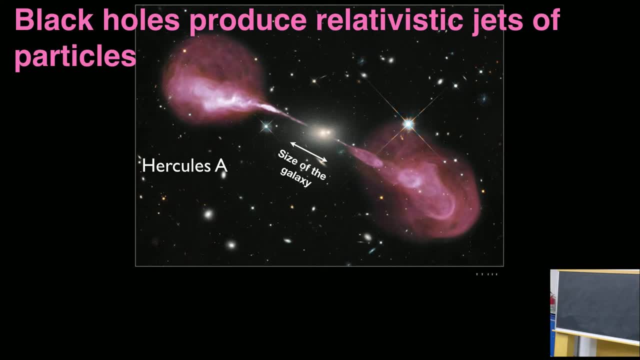 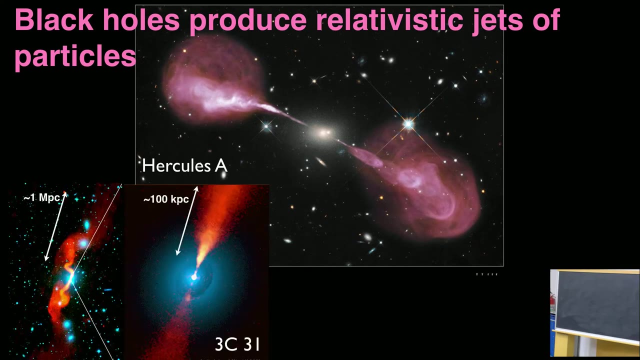 Look at the tiny size of the elliptical galaxy compared to the extent of the outflows coming from the center of the galaxy. This is not a model. This is a radio observation with a very large ray in New Mexico. This is another beautiful observation. 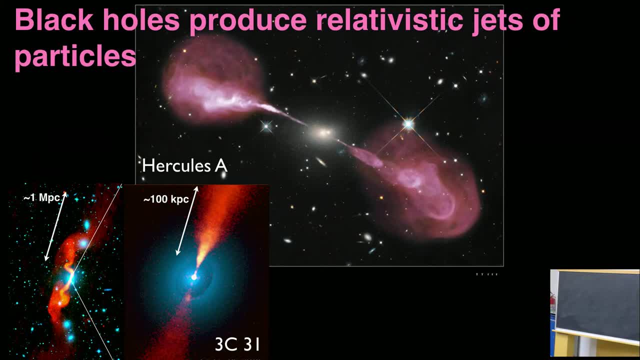 of a plasma beam being produced by the center of another radio galaxy called 3C31.. And here look at the tiny size of the galaxy, the collective emission of all stars in the galaxy, which was artificially colored as blue here, And look at how far the beam of plasma. 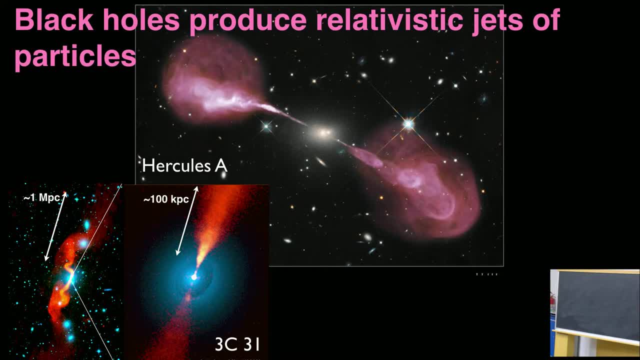 shoots out of the center of the galaxy. It goes up to almost five times the size of the, the size that you get from observing baryons in your galaxy. And look at this other image. You have now a radio galaxy with a phone number. 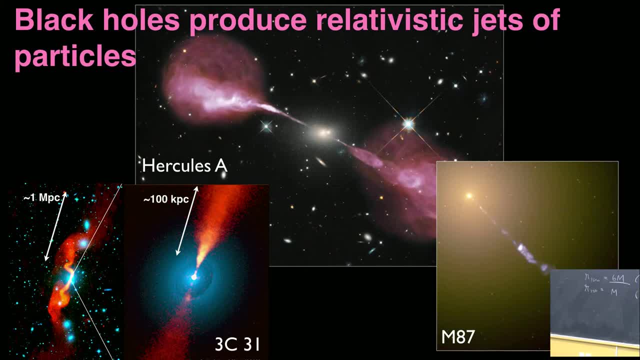 a Snapchat address of M87.. This is a particularly relevant target for astrophysicists, where again, there is something at the center of the galaxy shooting a very straight ray. We call these rays relativistic jets of particles, And this is reason to believe. 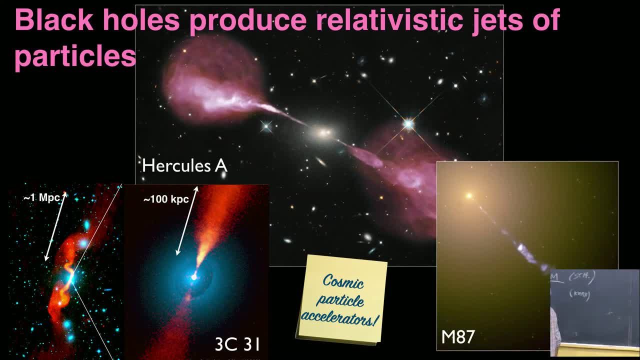 that there is something at the dynamical center of galaxies, of many galaxies, which are literally cosmic particle accelerators. So there is something which was mysterious but not mysterious anymore, that is shooting particles at the center of mass of a galaxy And when you go down, 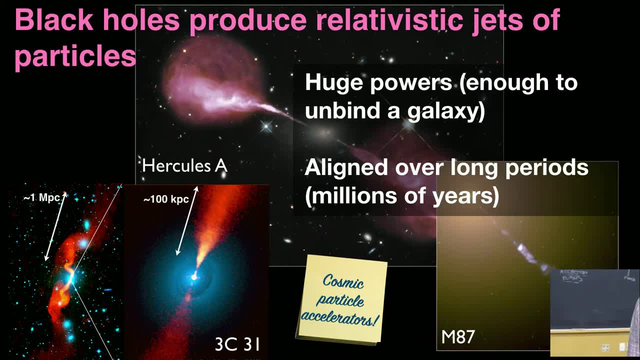 and you use some simple arguments to try to estimate the powers that are being carried in radiation, in kinetic energy. in momentum of these outflows, you derive powers, energies which are so big that if you were able to spread the power, the energy of this jet, 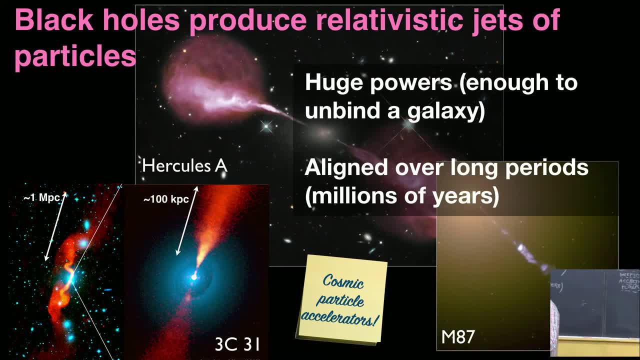 across all gas in the galaxy. you could invitationally unbind the galaxy. This is the kind of energetics we are talking about when we talk about these jets. So they carry enormous amounts of energy. Number one And number two: when you time particles take to cool down. 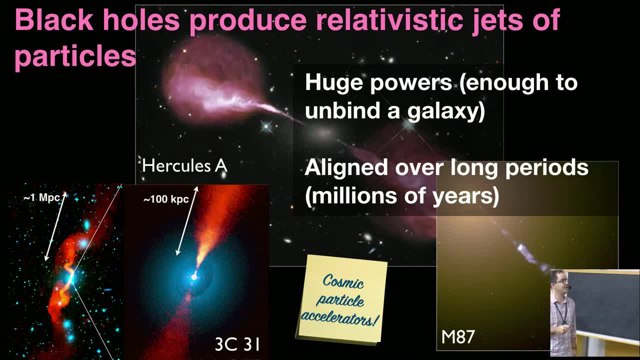 as they flow away from the center of the galaxy. you can have an idea of the age of these jets And you understand, we realize that the age of these jets- sometimes they are millions of years old, So there is something retaining the orientation of the rays. 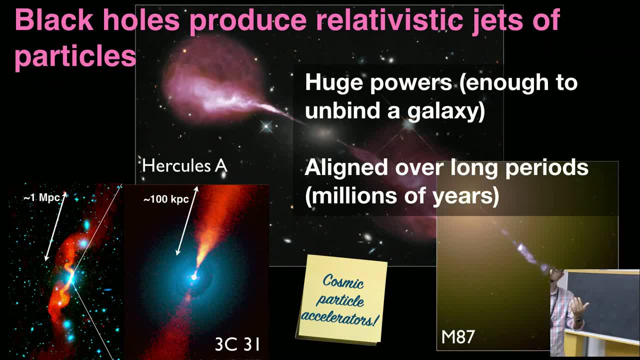 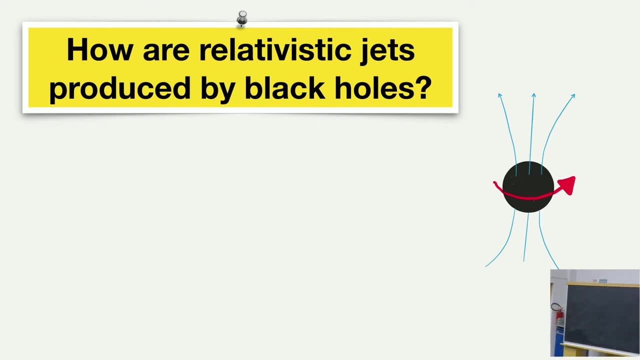 over millions of years And this is not easy. This is not easy unless you have a very powerful gyroscope to keep a line and power in this beam of particles over millions of years. So in the early 70s, the relativists 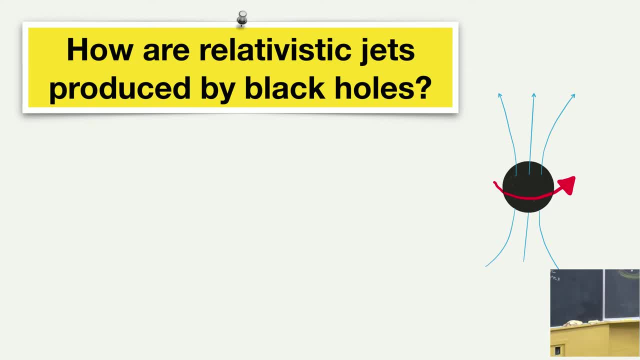 I don't know how to pronounce this word, but GR people, including Roy Kerr and other people which are now very famous, decided to sit together with astronomers and astrophysicists to discuss what could be powering these very strong rays coming from the centers of galaxies. 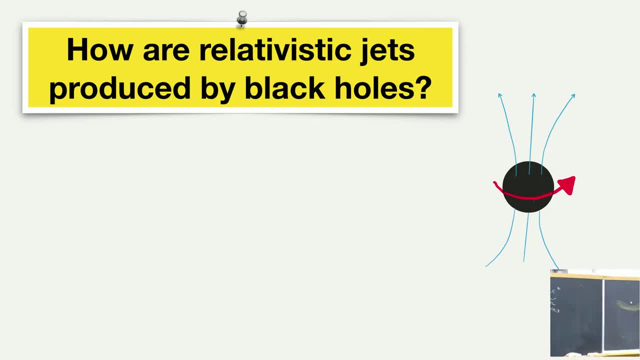 And they quickly realized that these jets, the most likely origin of the jets, is a black hole, More specifically, a Kerr black hole. This one is a conjecture. It still is a conjecture because we don't have a proof that these spinning black holes 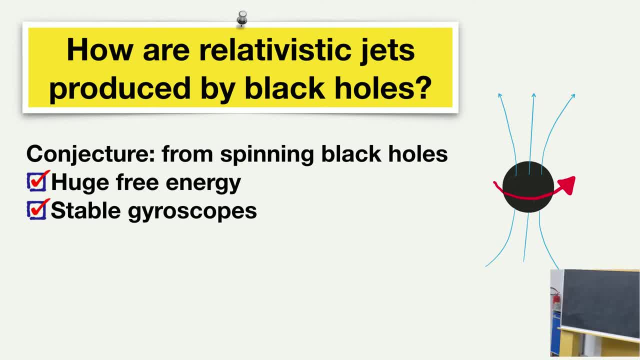 they are powering these relativistic jets. But the appealing things for theorists is that a spinning black hole has a lot of free energy in the rotating space-time that can be extracted by Penrose-like mechanisms And number two, Kerr black holes. they are very stable gyroscopes. 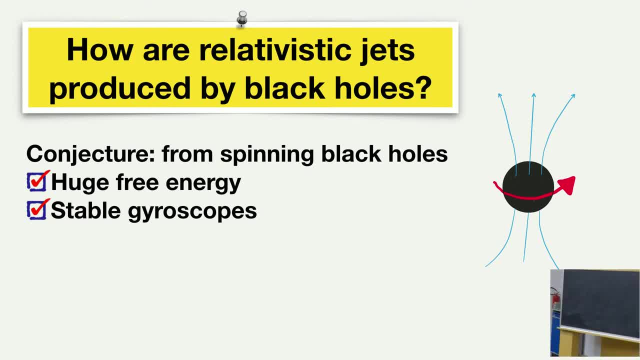 So the only one of the ways you can misalign the gyroscope in a Kerr black hole is if you throw another spinning black hole in a collision with this Kerr black hole, But this doesn't happen very often in astrophysics. okay, So from the very beginning, 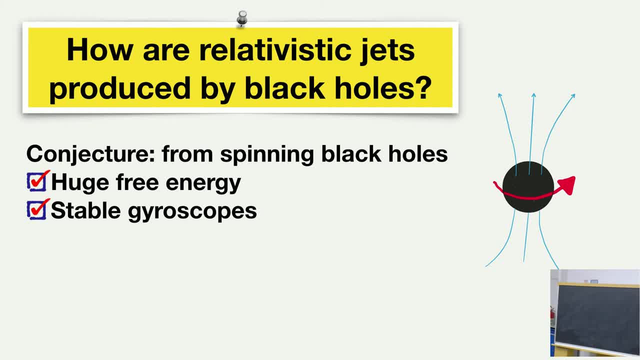 it was conjectured that spinning black holes could be powering these gigantic, beautiful relativistic jets, And there is growing evidence, growing empirical evidence, that this is in fact correct. There is no proof, but there is a growing body of evidence. Theory and simulation seems to agree. 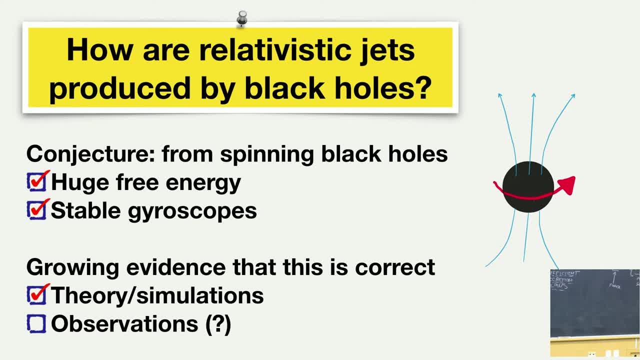 that there is a paradigm of spinning black holes, powering relativistic jets, but the observational evidence is that the observational picture, as usual, is way more messy and nonlinear, almost similar to biology, where you start building separate pictures until somebody figures out that DNA unifies everything. 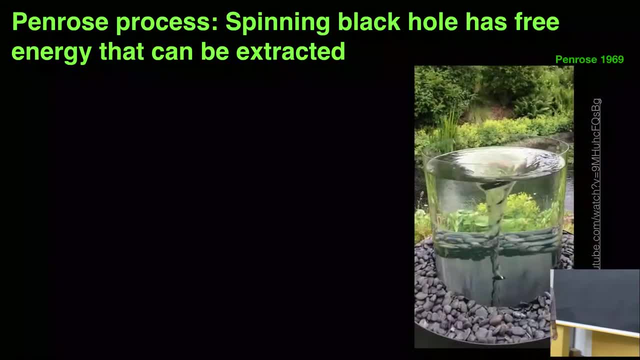 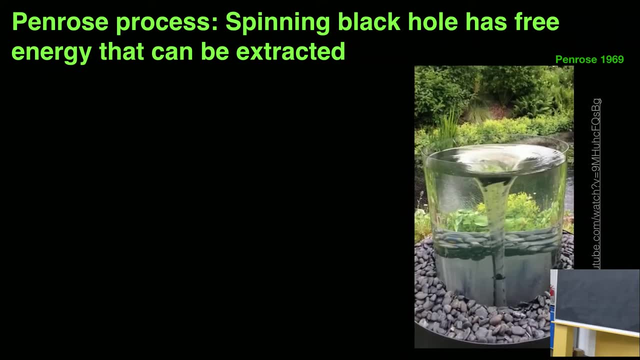 We are missing the DNA in astrophysics right now. So how can we extract energy from the black hole to power these very intense beams in relativistic jets? So Penrose, in the late 60s, proposed something called the Penrose process of extracting the free energy. 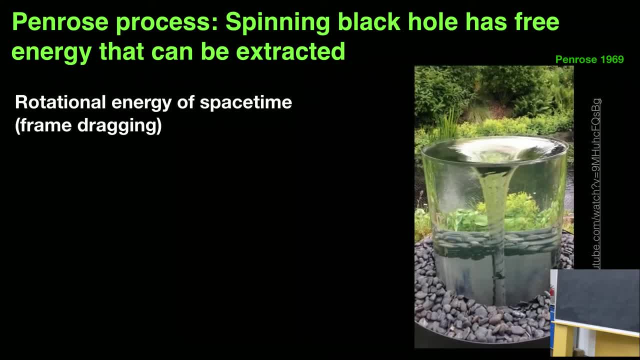 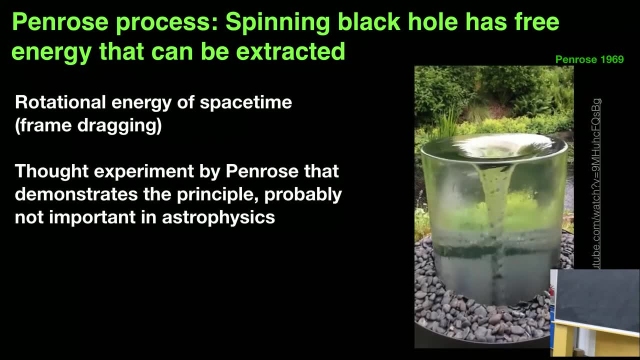 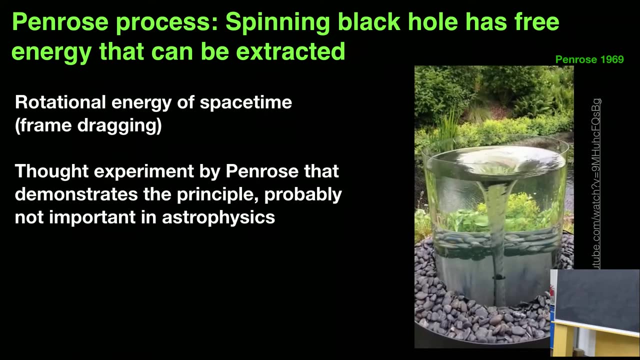 the rotational free energy of the Kerr black hole through exploiting the frame dragging around the spinning black hole. So this is a very interesting paper in the 1967 or 1969 by Penrose. But it was quickly realized that the Penrose process doesn't seem to be really applicable. 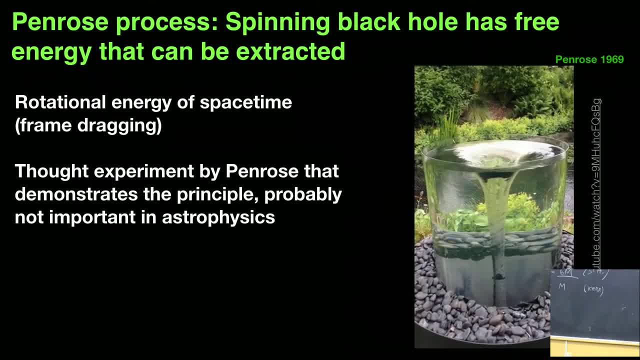 to astrophysics because you need to basically throw a projectile and destroy the projectile in the ergosphere and make part of the projectile, leave the ergosphere of the black hole and reach an observer. You have to fine-tune the orbits of your projectile. 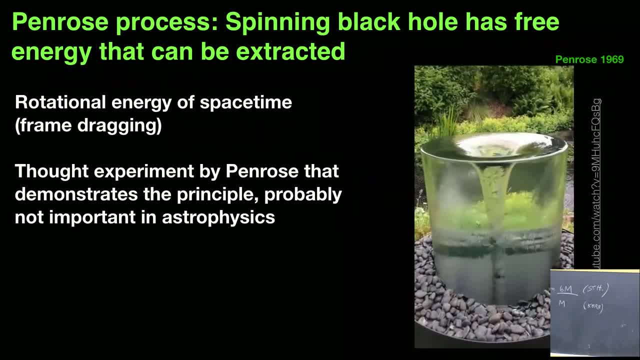 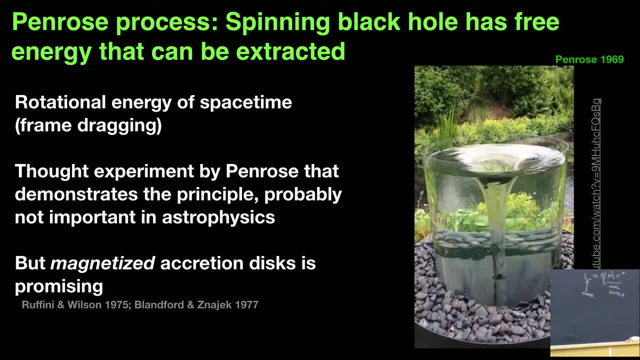 so it doesn't seem to be really easy to get energy with the original Penrose process proposed in the 60s. But there is a modified, updated, curable version of the Penrose process which seems to be relevant in astrophysics that I will mention now. 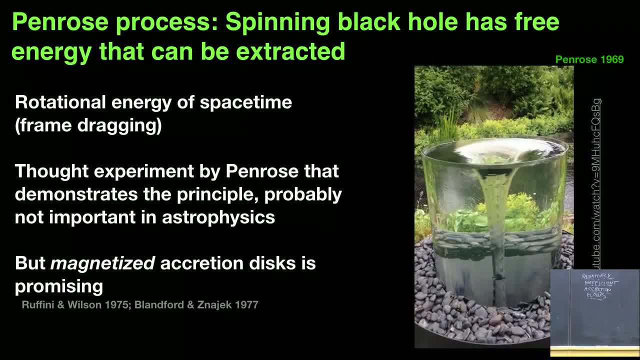 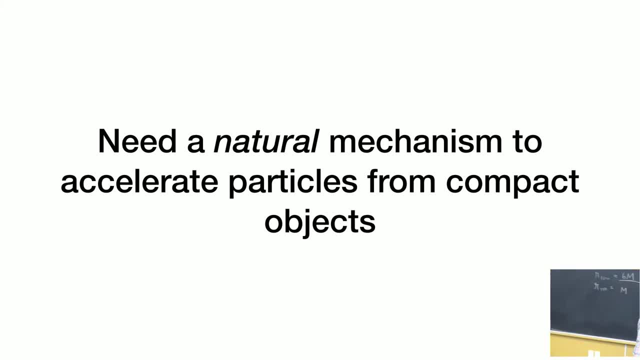 using magnetized accretion disks as agents for the Penrose process. But the bottom line so far of this presentation is that you need something that happens naturally. You cannot use some convoluted theoretical scenario because you see jets everywhere in the universe. 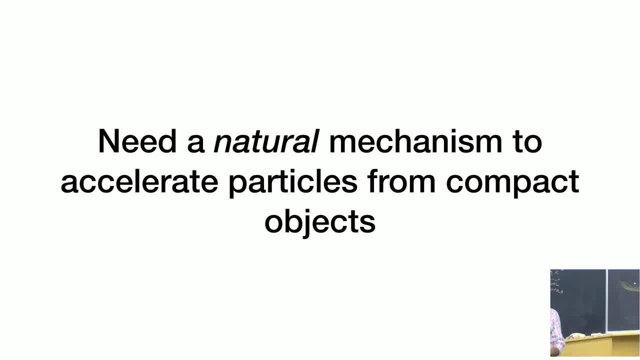 So this process that is powering jets, it must be something that you get reasonably easily from the evolution of galaxies and their central black holes, So you need something not so convoluted. Nature must be able to actually execute this process: energy from your black hole. 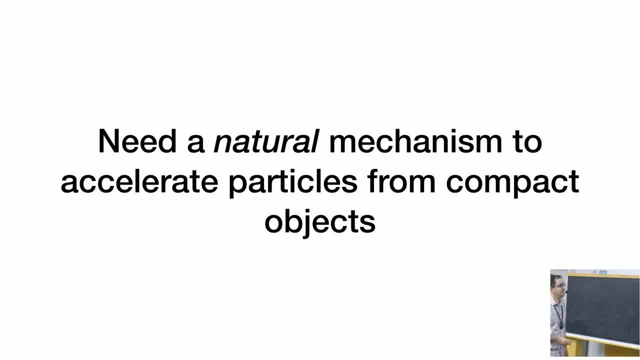 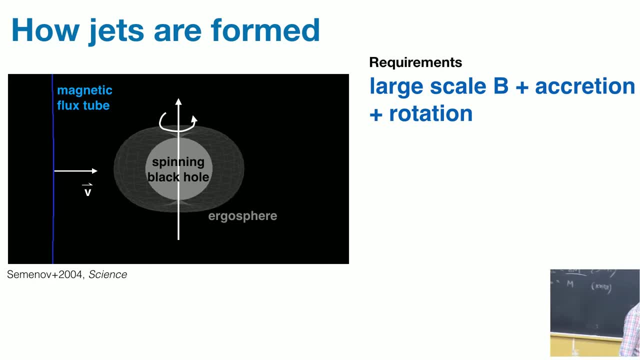 So what is the mechanism powering relativistic jets? So, after decades of work and, more specifically, numerical simulations of evolving Maxwell's equations in the curved space of curved black holes, we now have a very nice picture for how to get a cosmic particle accelerator with a curved black hole. 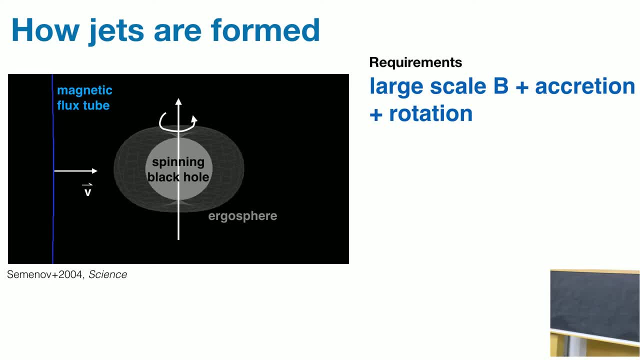 So the idea is the following. The idea is the basic ingredients for an astrophysical jet- is: you need a large scale magnetic field line, You need to bring this large scale magnetic field line close into the event horizon And you need rotation. So these are the three basic ingredients. 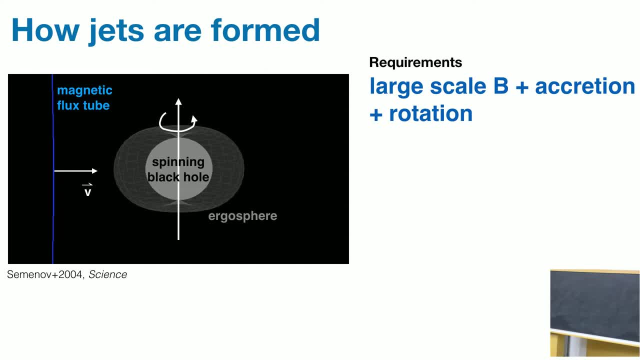 The projector is nervous to learn about the physics of jet production: It's trembling. So these are the three basic ingredients: Magnetic field, accretion disk and rotation. Large scale field, because this will be the agent of the Penrose process. 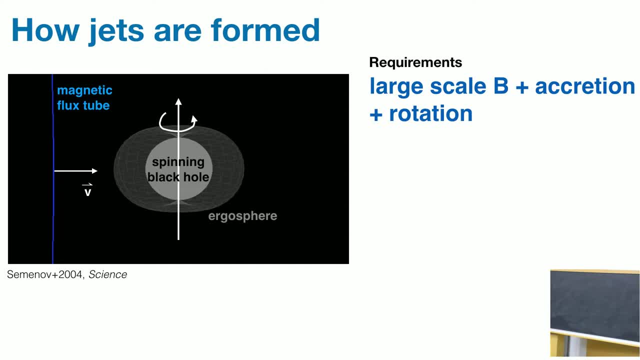 in astrophysics, Accretion- to bring the field into the ergosphere. And rotation, because we want to extract the rotation of the space time. So what I will show you now is a nice, clean numerical experiment published in a science paper 14 years ago. 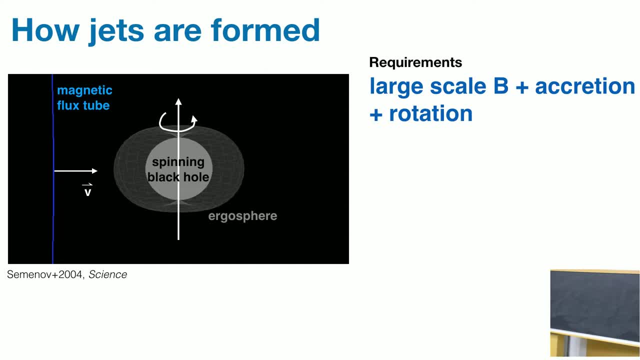 by a Russian physicist, Semenov- I don't know his first name- And what you will see here is a curved black hole In gray. you see the null surface of the horizon of the black hole. This is the ergosphere, where you cannot have static observers. 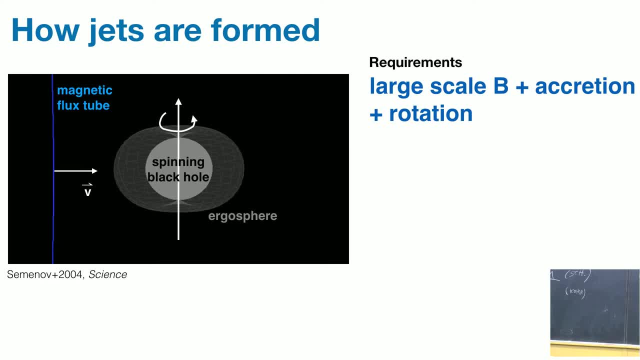 The strong frame dragging is happening inside the ergosphere And the blue line is a magnetic flux tube which will be moving and will be accreted towards the black hole. Look at the fascinating physics that will happen now as we play and solve the Maxwell's equation. 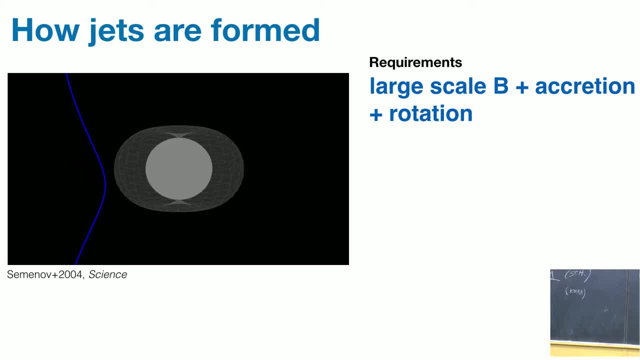 in the curved space time. So there is gas that is bringing the magnetic field into the horizon. The magnetic field swirls around the spinning horizon And what happens here? look at the number of loops that you have of azimuthal polar loops around the horizon. 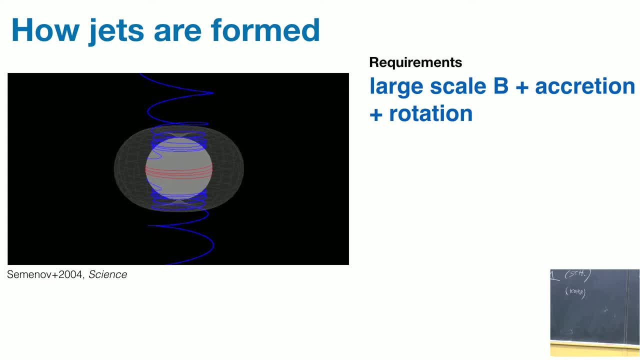 The frame dragging is making the field bend and create essentially a twisted tower of magnetic fields circling the horizon. As you can see, the angular momentum of the black hole is in this direction. I'm showing with my laser pointer And what happens here is that, as the frame dragging, 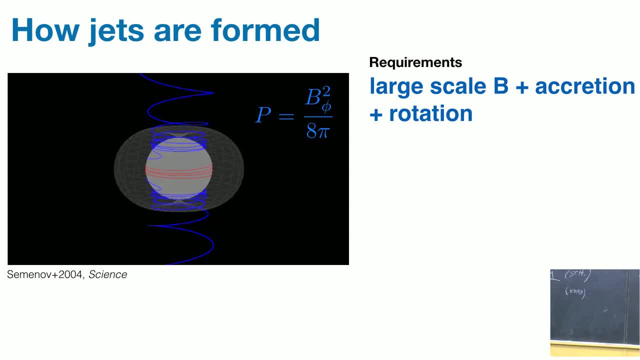 twists the magnetic field around the black hole, the pressure associated with it, the azimuthal component of the magnetic field, is growing. You are increasing the magnetic field, you are increasing the pressure, the magnetic pressure associated with the azimuthal, the phi component of the field. And if you study, 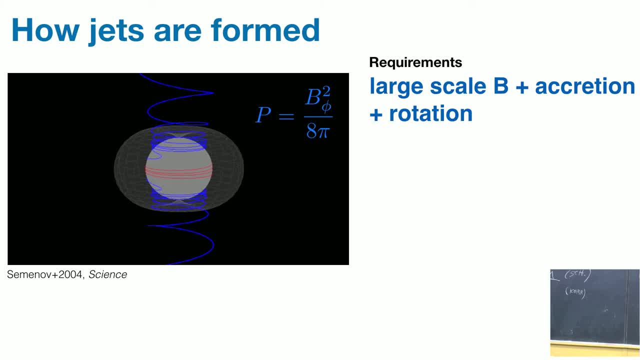 if you study electrodynamics, you know that one of the features of the dynamics of a magnetic field line is that few lines of the same polarity. they don't like to be close to each other. They want to get farther away from each other If you try to bring them close together. 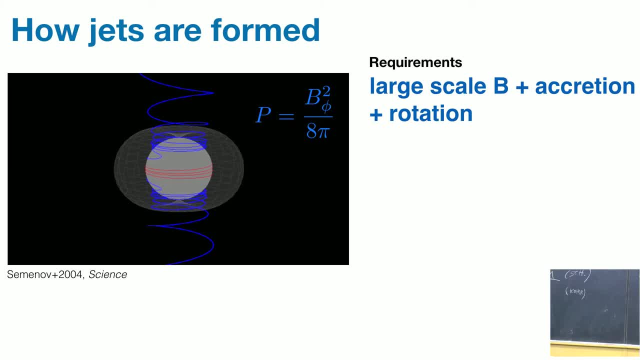 they're like: oh, I don't like you. You have the same polarity as I have. I don't like you. go away. So this is what's happening here. You are increasing the pressure here. What do you expect to happen? 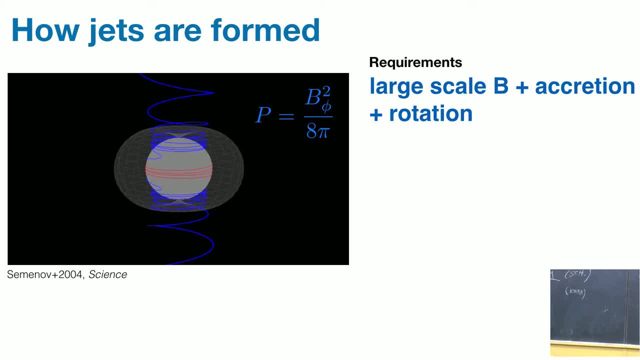 You expect them to be thrown away because they don't like they have the same polarity, they don't like each other. What happens next? The built up phi pressure, the phi component pressure of the field, creates a twisted tower of magnetic fields that will bring together 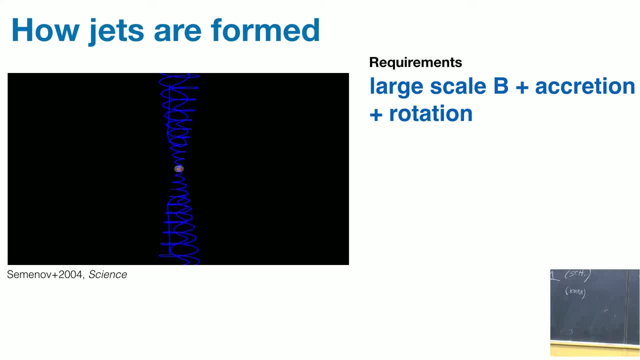 with this extraction, any charged particle that is forced to move along the magnetic field. This is the mechanism for producing a jet: Very easy: no extra dimensions, no charged black holes, no fancy things. this isn't a more likely version of the Penrose process. you just need: 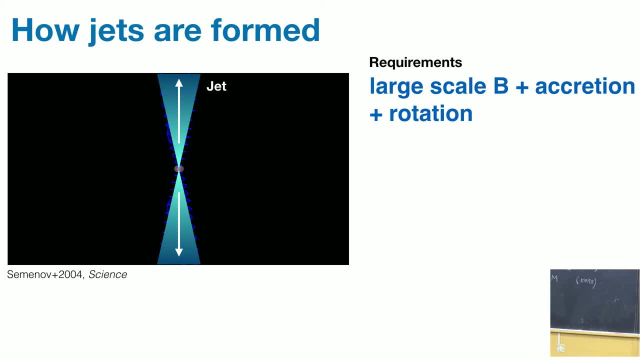 B, accretion and rotation and you get a cosmic particle accelerator. This mechanism is nowadays called in astrophysics Blanford's magic process in honor of Roger Blanford, who is now the director of astrophysics in Stanford. and this guy Romans and became the mayor. 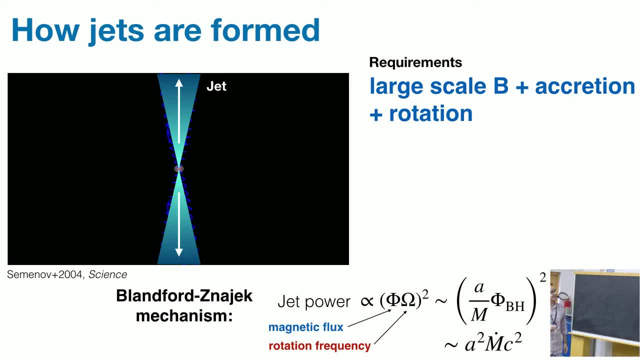 from a small town in England, but they published in 1977 a seminal paper where they solved a perturbative version of Maxwell's equations in a slowly spinning curve, a slowly spinning black hole, and they demonstrated that- the jet power, you get out of this cosmic. 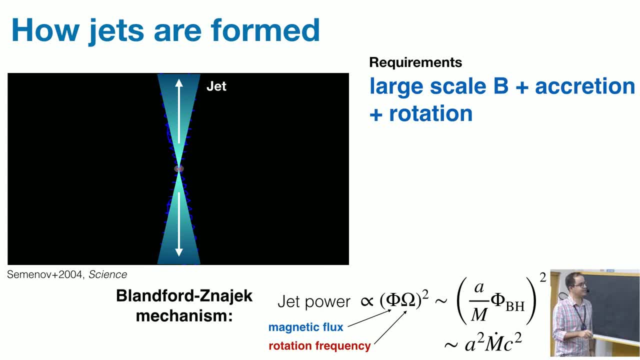 literally, cosmic battery is proportional to the magnetic flux that you bring close to the horizon, times the rotation frequency of the horizon to the square power. you can't demonstrate this in different ways. this expression, it could even be a homework to you guys and then you put in the physics.